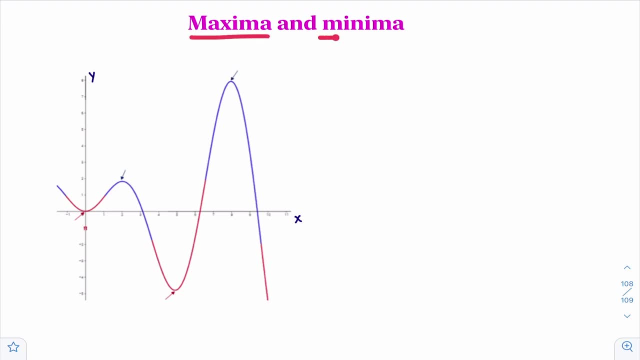 Applications of derivatives. Maxima and minima. This is the last concept in applications of derivatives. Those who already understand increasing function and decreasing function, they can understand this very easily. To avoid unnecessary confusion, I don't want to explain all the things. what is there in the textbook? I find out that so many students they feel. 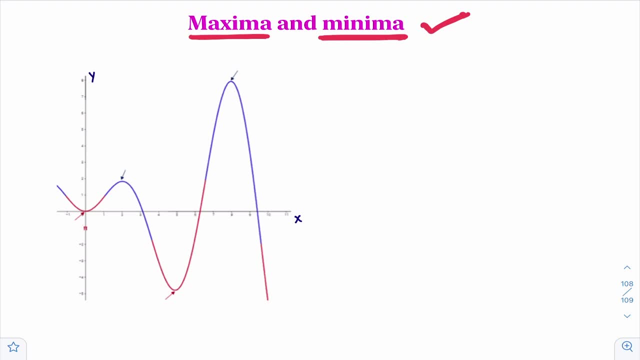 difficult while learning maxima minima. Actually, maxima minima is very easy if you are good in the concept Here you observe: I considered a graph. I considered a graph. This is that graph. This is the function f of x. The function is like this: This is the graph. I taken What you observed by. 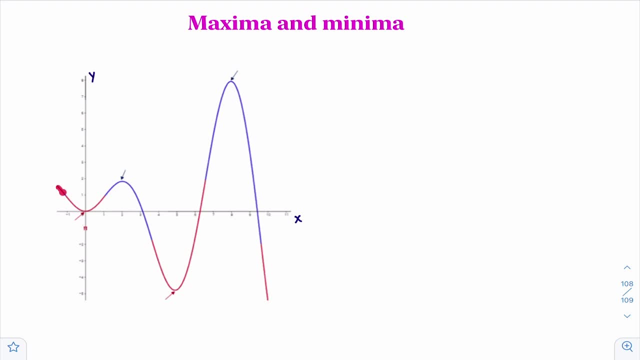 seeing the graph, You see this function is decreasing, decreasing, decreasing. At this point onwards. this is started increasing At this point onwards. this is started increasing Right, Very good. So you see, now this function is increasing, increasing From this point. 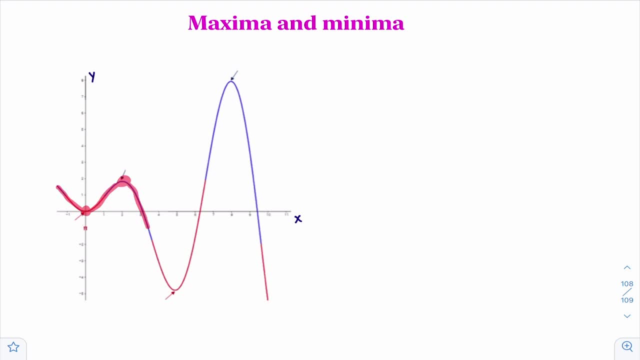 onwards, the function is started decreasing Right, Like that you observe here. these are the points which plays important role. These points are known as critical points. These points are known as critical points. Why these points are critical points? At this point, the function attains either: 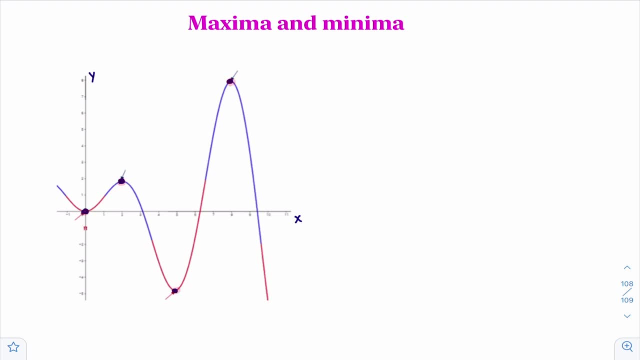 maximum value or minimum value. At this point, the function attains either maximum value or minimum value. You observe here, you observe this point and this point, At these points, the function f of x. This is the function. This function attains minimum value. You observe at these points the function. 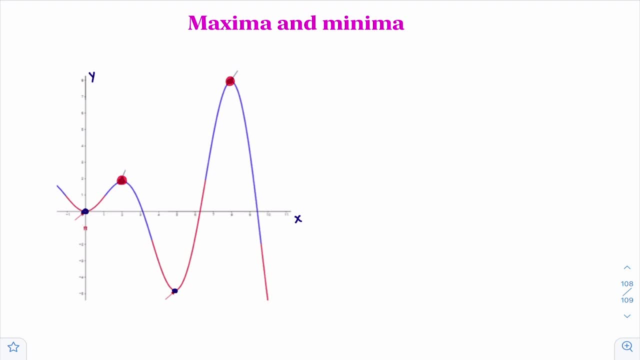 attains maximum value And what these points are known as. These points are known as critical points. So you learn about critical points. What are critical points At these points? the function attains either maximum value or minimum value. And you can observe one more thing At these points. 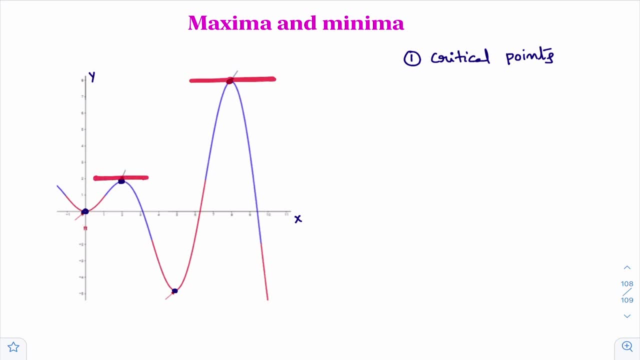 if you draw the tangent, you observe at these points, if we draw the tangent, the tangent is parallel to x-axis, Whether it attains maximum value or minimum value. you can observe. These are the tangents to the graphs at the critical points. If we draw the tangents to the graph, 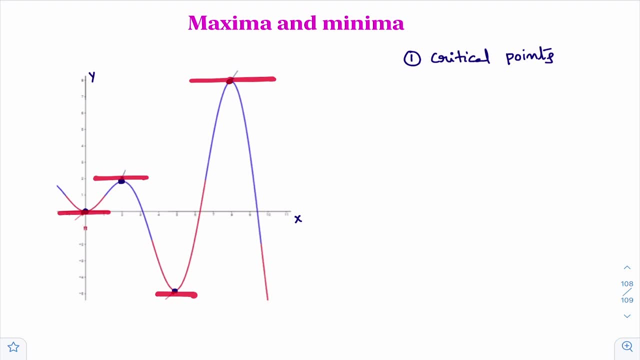 at the critical points. the tangents are parallel to x-axis. I hope you are understanding Here by using this concept. the tangents are parallel to x-axis at the critical points. By using this concept I can find critical point Here. you know, from tangents and normal chapter you know that. 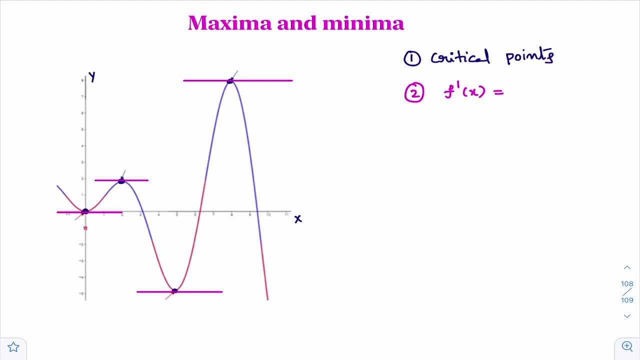 f dash of x is slope of the tangent. From tangent and normal concept we learn this: f dash of x is slope of the tangent. So if the tangent is parallel to x-axis, what is slope of x-axis? In straight lines chapter we learned that slope of x-axis is the slope of the tangent. 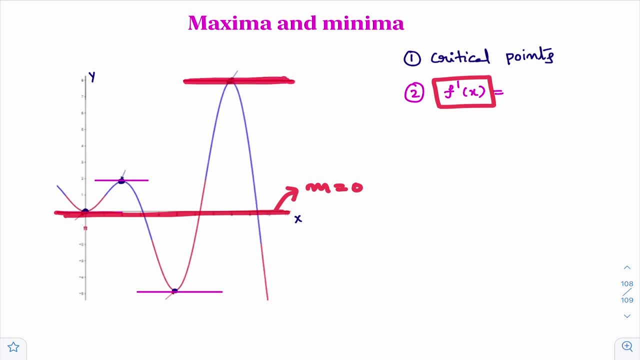 Here this tangent is parallel to x-axis. Slope of a tangent which is parallel to x-axis is also zero. We know that f dash of x will give you slope of the tangent. So how to find the critical points? First, you differentiate the given function. You observe this is the given function f of x. 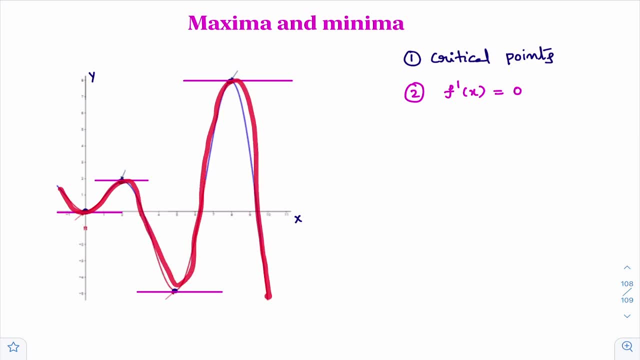 You differentiate this function, They will give function f of x. You differentiate it and equate it to zero. For what values of f? dash of x is zero? For what values of x? f dash of x is zero? those x values will give you the critical points Those x values will give. 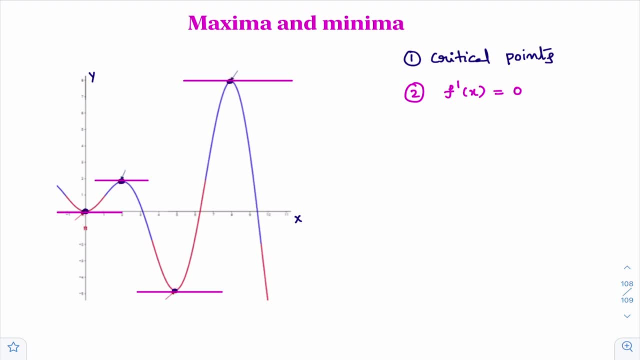 you the critical points. Once you know x value, then you can find y value also Here now you learn about critical points and how to find the critical points. That also you learn Now. third point: What is meant by local maxima, local minima, absolute maxima, absolute minima? Many students 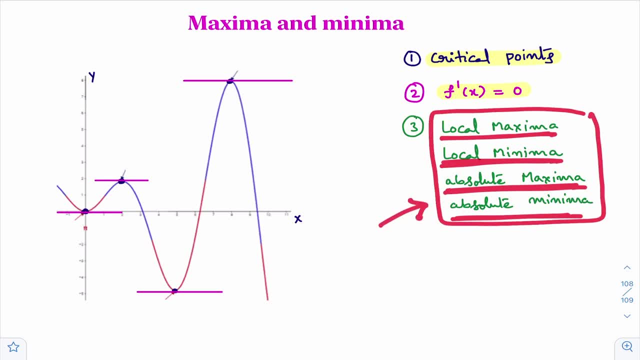 confuse with these words. We use these words very frequently while solving the problems. Now I will try to explain. what is local maxima? what is local minima? what is absolute maxima? what is absolute minima? You observe, this graph attains minimum value at these points. Please, 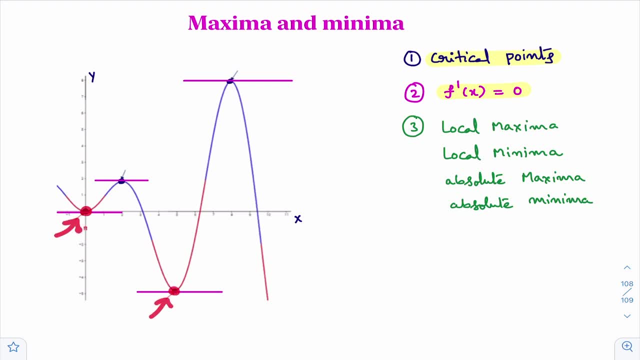 observe, this graph attains minimum value at these two points. If I consider this function, if I consider this function here, these two are the points, At these points the function attains minimum value. Actually, this point, this first point, is there. Look here this point. 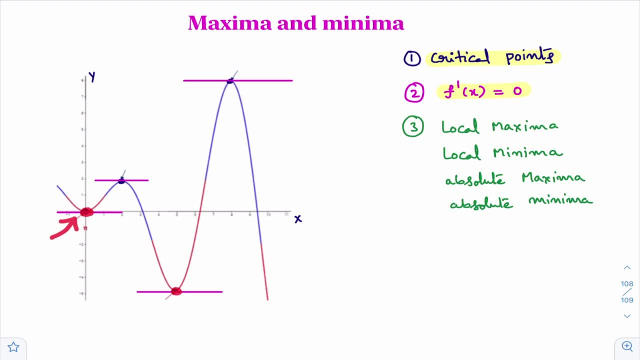 This is attains minimum and at this point also function attains minimum value. In these two, which one is a more lesser value? That means this one. You observe this is negative value. you are getting right. So this is zero. you are getting Here what I am trying to say. 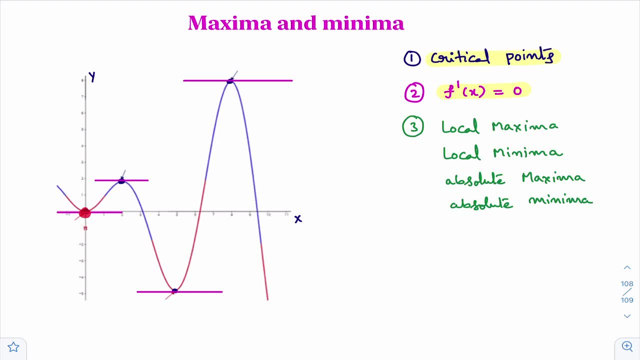 this point, I will call it as local minimum and this point, I will call it as absolute minimum. I try to understand this point is what This point is local minimum and what is this point? This point is absolute minimum. So you learn what is local minimum, what is absolute minimum. 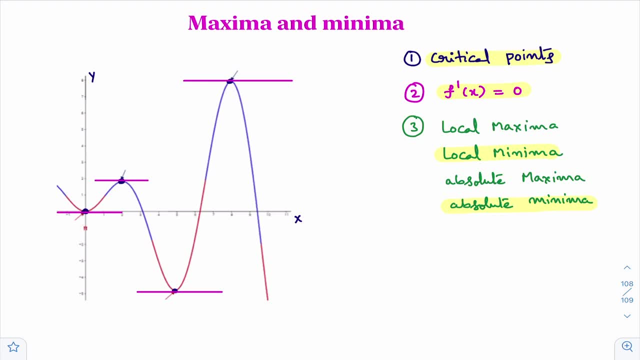 right Now. you observe the graph Here. at this point, this function attains maximum value. At this point also, the functions attains maximum value. In these two values, which one is the greatest value? You see, this is smaller when compared with this number. 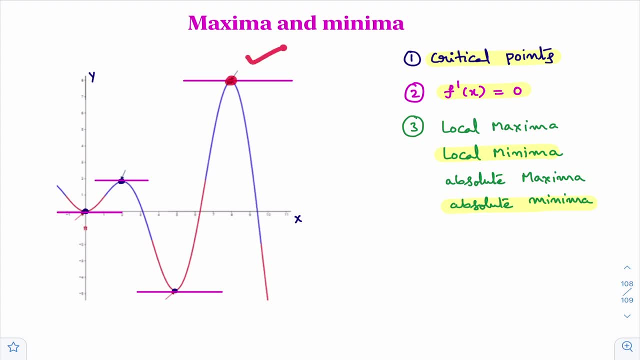 So this is the absolute maxima. this is local maxima In this graph. by considering this graph, I am explaining right. This is what. This is local maxima. What is this? This is absolute maxima. That means, if you observe this entire graph, maximum value is there here. This is the. 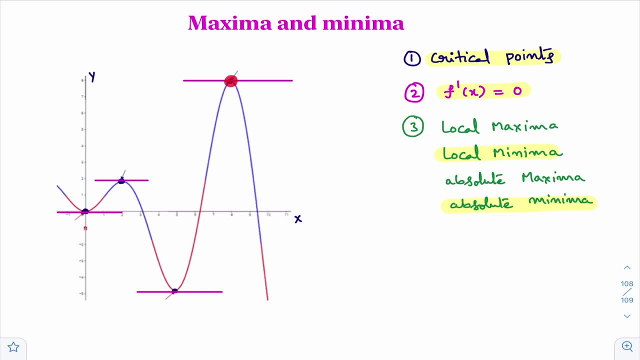 maximum value. That's why this is called absolute maxima. You can observe, this is also one maximum value. It is not absolute maximum value. That's why this is called local maxima. I hope you are understanding Here. absolute maxima is also known as global maxima. I hope you understand what is. 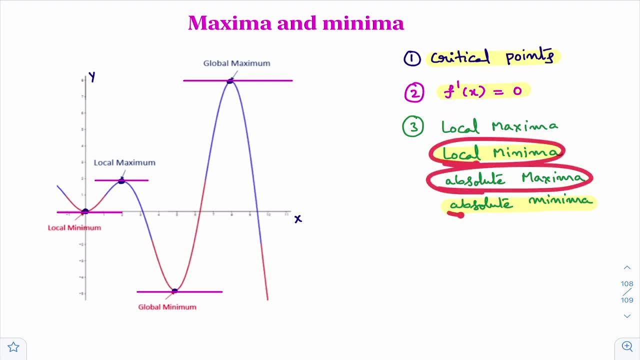 local maxima, what is local minima? what is absolute maxima, what is absolute minima? Now you see what is first derivative test, what is second derivative test. Throughout this chapter we will try to find where the function is maximum, where the function is minimum. Throughout this, 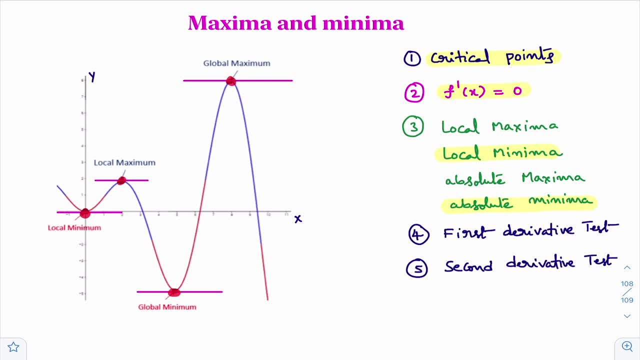 chapter. we will try to find where the function is maximum. where the function is minimum, what is that maximum value? what is that minimum value? We will try to find those things throughout this chapter To find where the function is maximum. what is its maximum value. where the 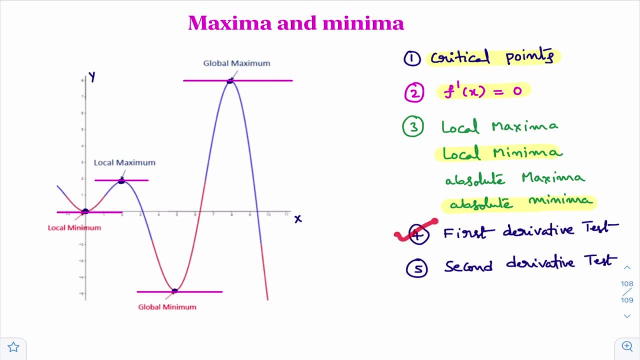 function is minimum, what is its minimum value? we will use two tests: First derivative test, or we can use second derivative test also. So first we will learn what is first derivative test and what is the working rule, And to identify where the function. 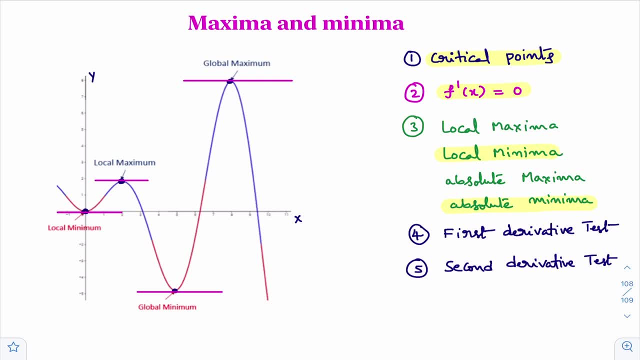 is maximum, what is its maximum value? where the function is minimum, what is its minimum value? we can use second derivative test also For most of the problems in this exercise. we will use second derivative test only Because by using second derivative test most of the times we can. 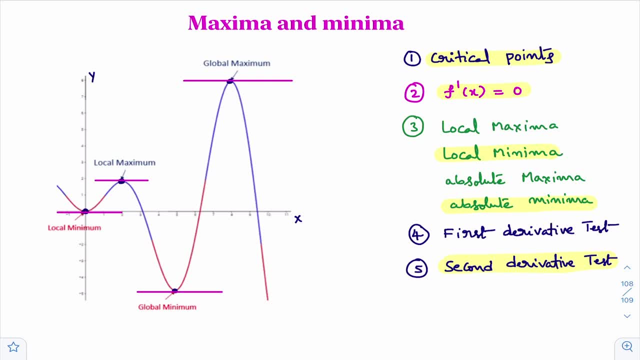 find where the function is maximum, where the function is minimum, easily when compared with first derivative test. Second derivative test is easier when compared to first derivative test. That's why for most of the problems we will use second derivative test only. It is not compulsory. 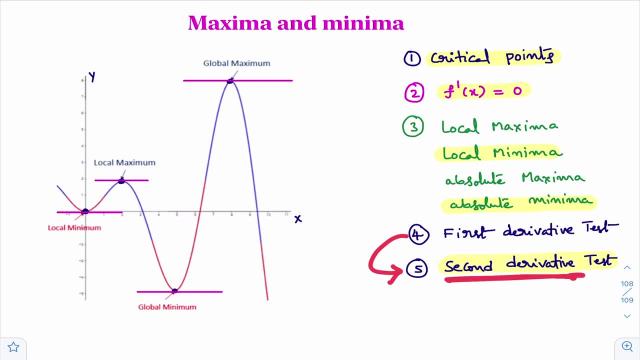 you need to use second derivative test. for most of the problems, You can use either first derivative test or second derivative test. Our intention is to make the things are simpler. That's why, in this exercise, most of the problems we will solve by using second derivative test. 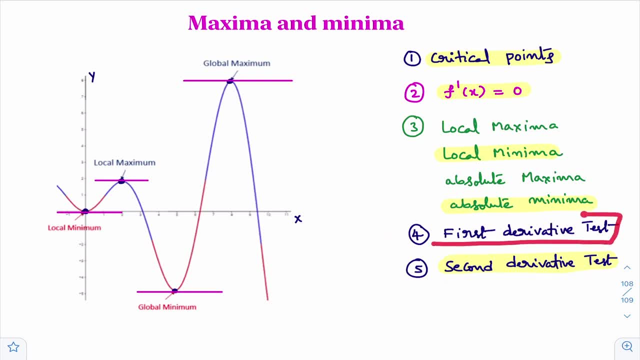 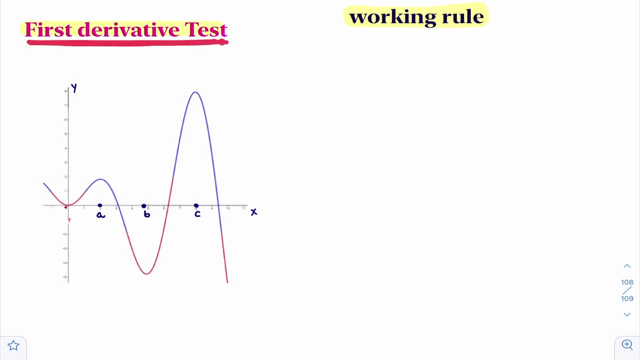 Now we will learn what is first derivative test. What is first derivative test? By using first derivative test, we can identify where the given function attains maximum value or minimum value and what is the maximum value of that function and what is the minimum value of that function. 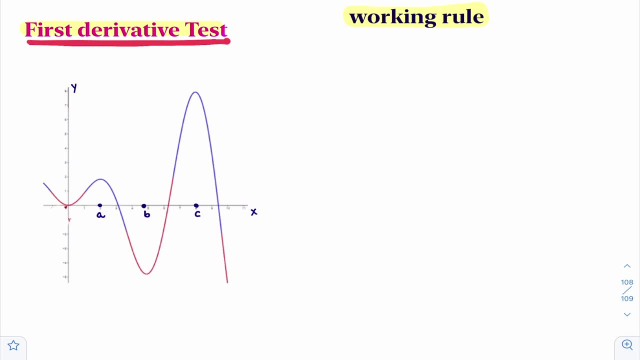 These things we can calculate by using first derivative test In this. now we are going to learn what is the working rule. first to eyes: used first derivative to test to identify where the function attains minimum values, where the function attains maximum values. First point: when we use first derivative test, 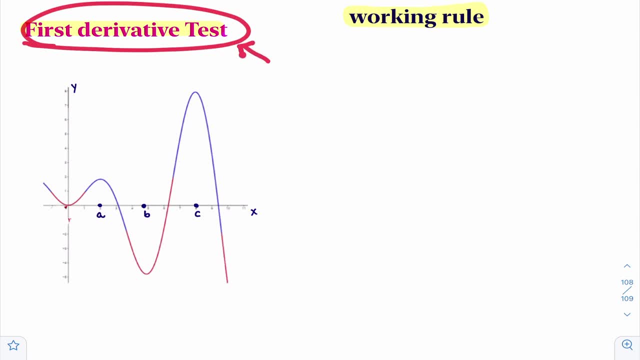 to identify where the function is maximum or where the function is minimum, how to find what it is maximum value and what is its minimum value. To identify those things we will use first derivative test. What is working rule? First step: which function- maximum values, minimum values you want to find, you take 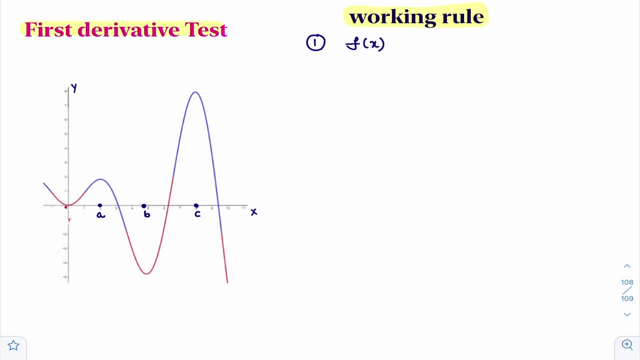 that function as f of x. Which function maximum values, minimum values you want to find. you take that function as f of x Here. this is the function f of x In this graph. this is the function f of x. 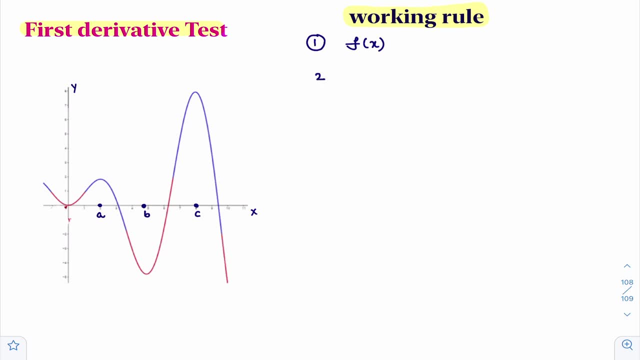 Okay, After considering f of x, you just calculate f dash of x. You calculate f dash of x. You know how to calculate derivative of a function from differentiation. You calculate f dash of x. After calculating f dash of x, you observe, we learned about critical points. 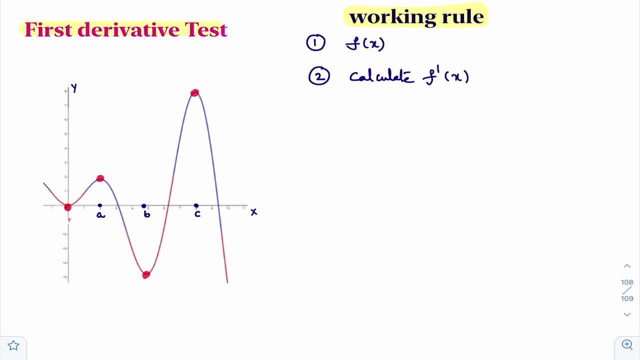 At these points the function attains either maximum value or minimum value. You need to find these points. You know, at these points, if we draw the tangent, the tangents are parallel to x axis. So to find these points, to find these points right, what I will do, 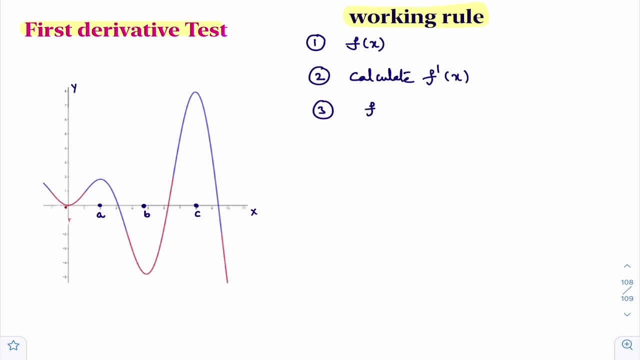 I will equate f dash of x to zero. You equate f dash of x to zero and solve this. If you solve this, then you will get x values. For example, I will take x values are a, b, c, something like that. you will get. 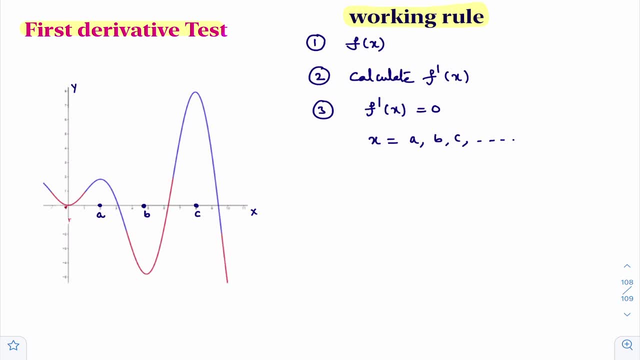 You will get one or more than one value right. So first thing is, what? For which function maximum minimum values you want to find? you choose that function as f of x. After that you differentiate that function and you will get f dash of x. 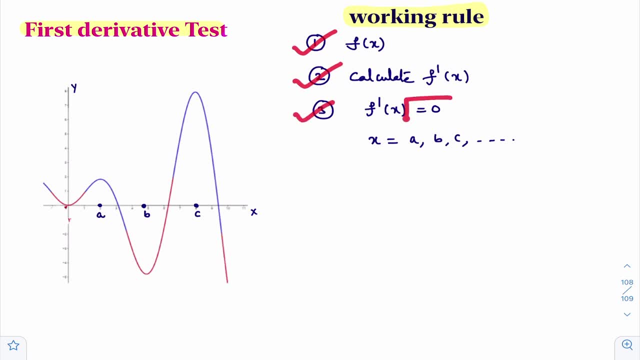 After calculating f dash of x. Okay, You equate that to zero. You equate f dash of x to zero and you solve this equation. Then you will get x values. You observe here: at this point, function attains maximum value. 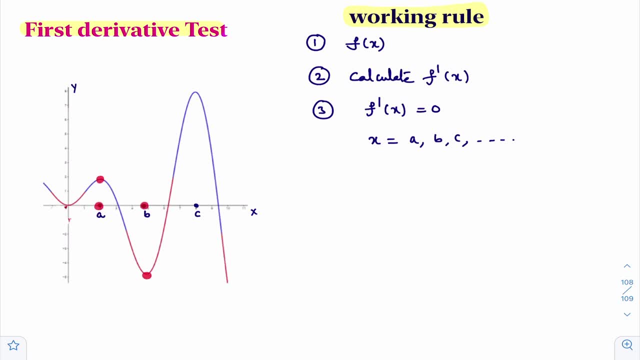 This is critical point: A value you got At this point, function attains minimum value. So you got b value At this point, function attains maximum value. Those values critical values. you will get, Okay, After calculating these critical values, what to do. 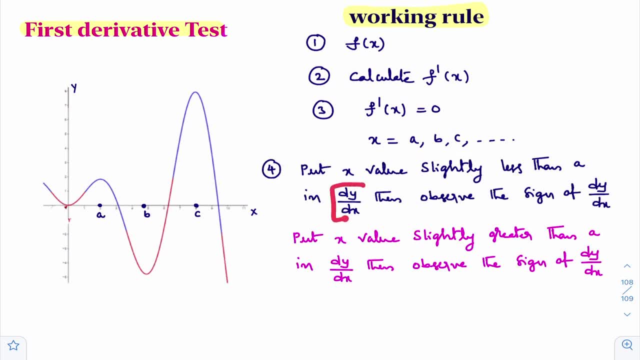 This is important. Listen carefully Here. dy by dx means what? dy by dx means derivative of the function f, dash of x. You observe, here put x value, which is slightly less than a. You see here this is x value. 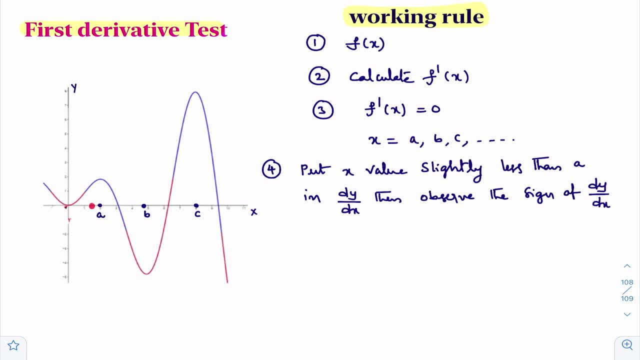 You take slightly less than a, slightly less than a. You put x value slightly less than a in dy by dx. For example, if you suppose this is 1, you take 0.9.. You take 0.9, substitute that in dy by dx. 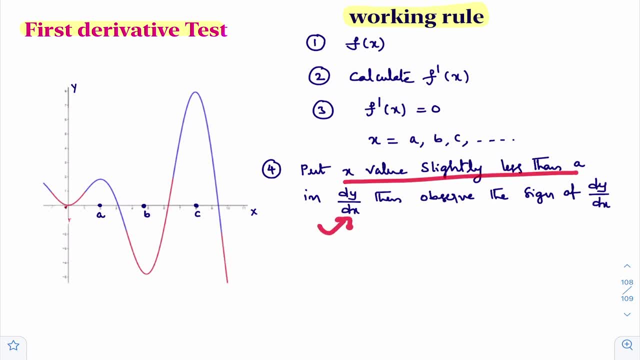 Put x value, which is slightly less than a, in dy by dx And observe here, Observe this sign of dy by dx. Sign of dy by dx means you observe that after substituting that x value, which is slightly less than a, you observe that dy by dx is positive or negative. 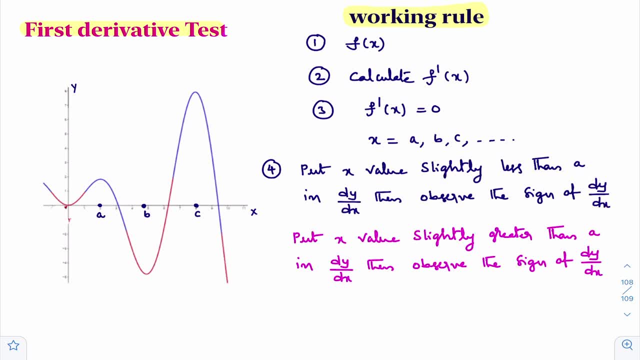 Just observe this sign. Okay, And you keep that in your mind. Again, put x value which is slightly greater than a. Earlier what we did: we substituted x value which is slightly less than a in dy by dx. Now you take x value which is slightly greater than a and substitute in dy by dx. 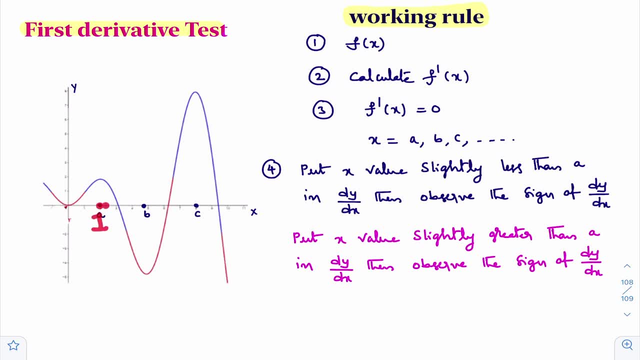 For example, this is 1.9.. This is 1.. You suppose this is 1.. You take 1.1, slightly greater than 1, and substitute in dy by dx and observe the sign of dy by dx. Just keep in mind dy by dx is positive or negative. 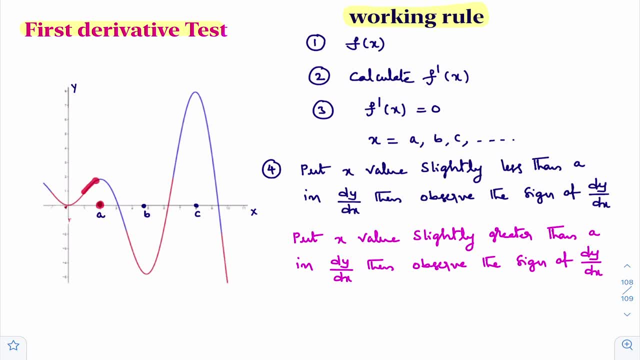 At this a. in this particular graph, the function attains maximum value. right At a. the function attains maximum value Here if I take a value which is slightly less than a. at that point, if I draw the. 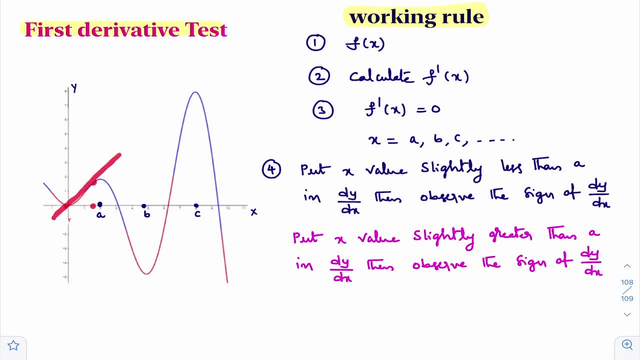 tangent. you draw the tangent at the point where a is less than a, x value is slightly less than a. You can observe, this makes acute angle, This makes this line makes acute angle. This tangent makes acute angle with x axis. We know that, dy by dx, we know that dy by dx, dy by dx is nothing but slope of the tangent. 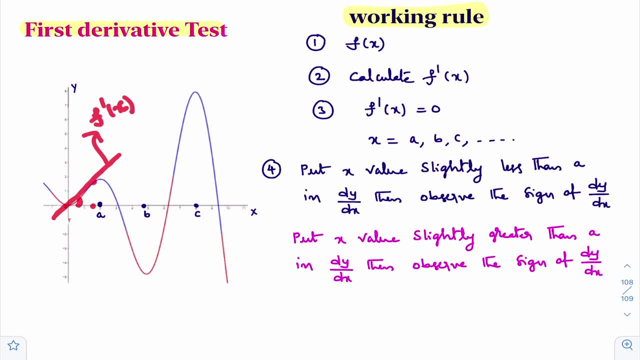 Slow dy. f dash of x is slope of the tangent. Here this tangent makes acute angle, So slope of the tangent. If theta is acute, that means theta lies in first quadrant. F dash of x. F dash of x will gives you slope of the tangent. that is tan theta. 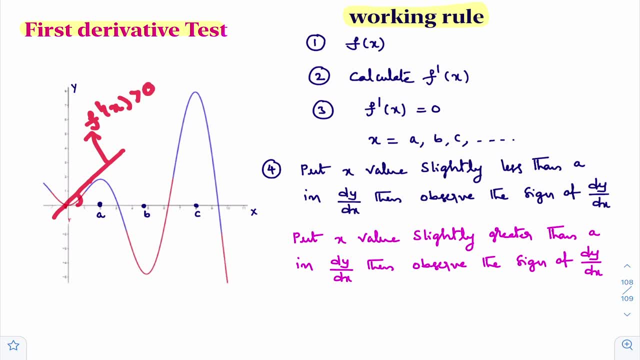 In first quadrant tan theta is positive. now f dash of x is greater than zero If the function attains maximum value at x equal to a. when we put x value slightly less than a, f dash of x is positive. At the same time you draw the tangent at the point where x is slightly greater than. 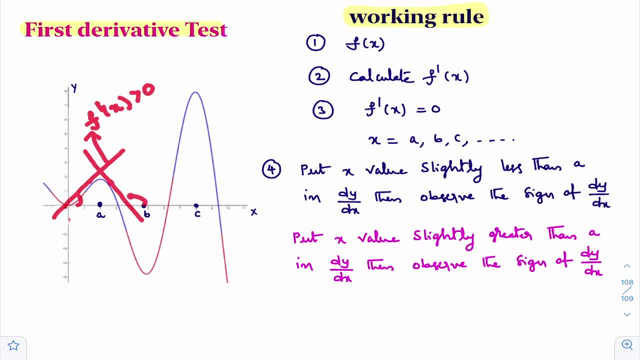 a. You draw the tangent at this point You can see that this is obtuse angle. see greater than 90 degrees. I hope you can understand. This is obtuse angle. Obtuse angle means slope of the tangent is negative. Slope of the tangent is negative. 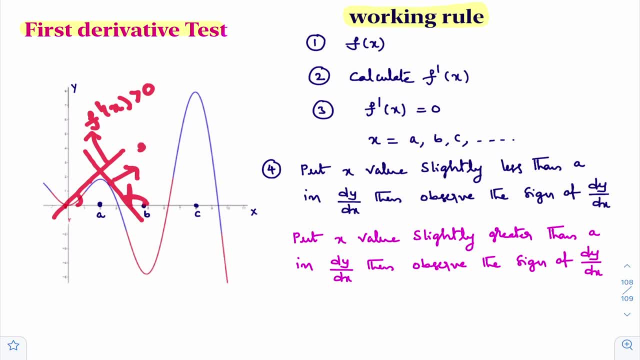 Obtuse angle means in between 90 to 180 in a second quadrant. In second quadrant, tan theta is what Tan theta is negative. So what you identified, dy by dx, changes the sign from positive to negative when it attains maximum value. 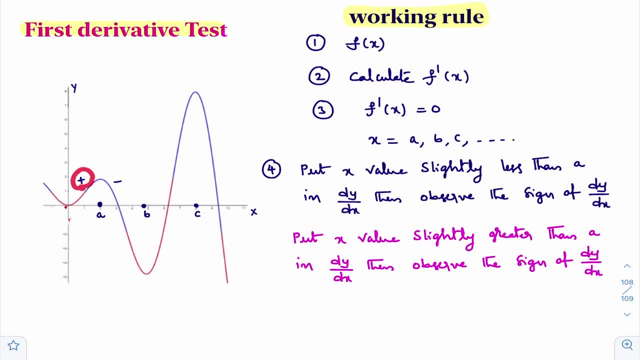 I hope you are understanding this. You observe dy by dx changes its sign from positive to negative when the function attains maximum value. When you substitute x value which is slightly less than a, you observe the sign of dy by dx. You suppose that dy by dx is positive. 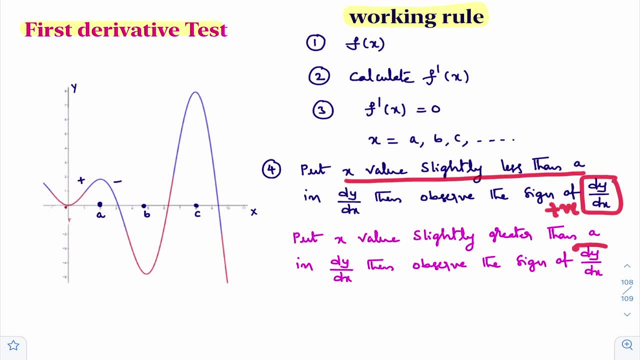 Suppose you suppose dy by dx is positive and you are observing the sign. You suppose that when we substitute x value slightly greater than a dy by dx is negative. What happened? dy by dx changes from positive to negative. If dy by dx changes from positive to negative, we can say that function attains maximum value. 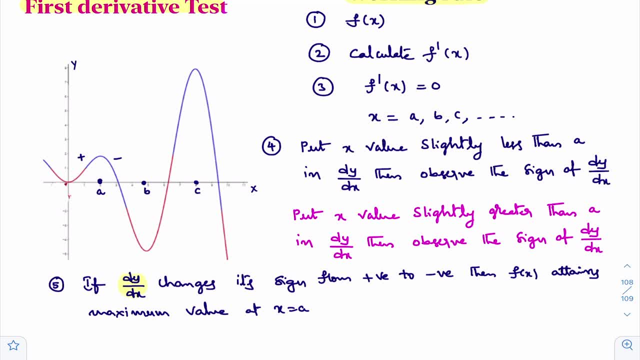 at x equal to a. You observe, I written the same thing. dy by dx changes its sign from positive to negative. Then f of x attains maximum value at x equal to a. And what is the maximum value? Maximum value is f of a. 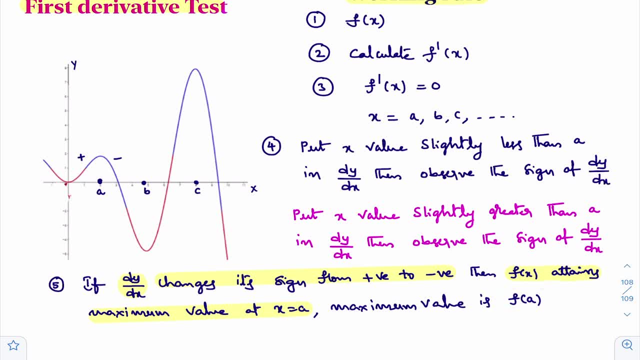 The maximum value is f of a. In the same way you observe at b in this graph, the function attains minimum value. So you see here, if I draw the tangent, if I take x value which is slightly less than a, and if I draw the tangent at that point the tangent makes Aptus angle. 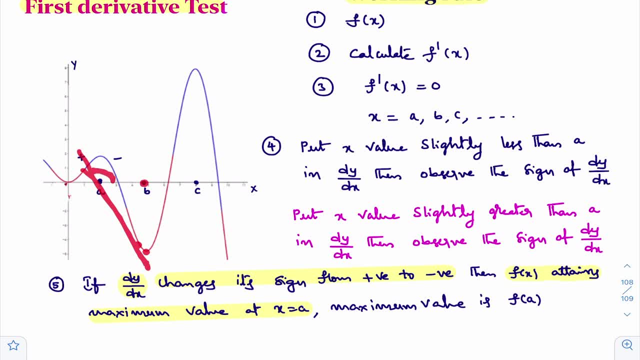 If the tangent makes Aptus angle means slope of the tangent. f dash of x is negative. f dash of x is negative And you take x value, which is slightly greater than b, and draw the tangent, at that point you can observe that this makes acute angle. 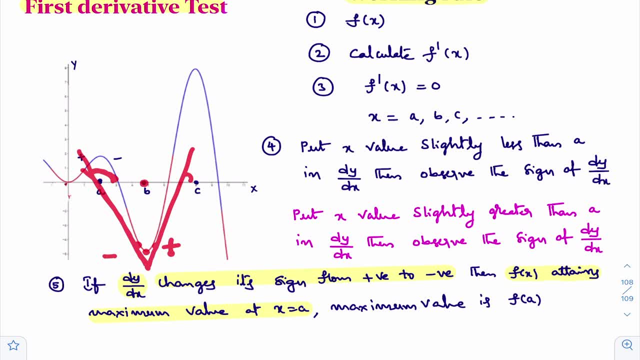 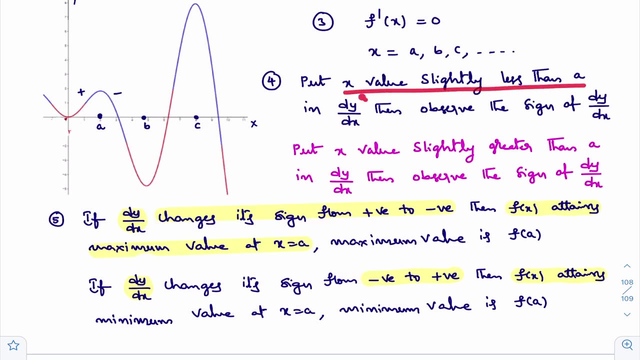 That means slope of the tangent is positive. So if dy by dx changes its sign from negative to positive, then the function attains minimum value. This is the example I explained at b. This may happen at a also, As you substituted x value slightly less than a in dy by dx. you are observing the sign. 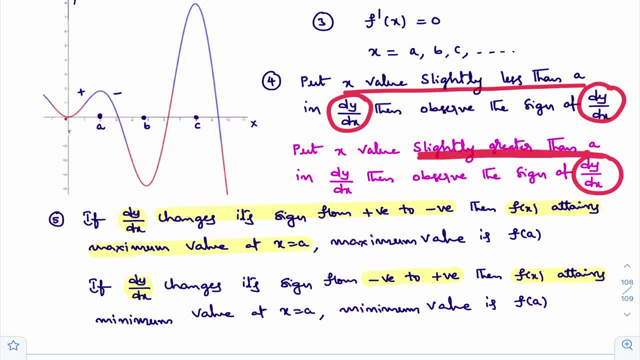 of dy by dx, as x value is slightly less than a, as well as x value is slightly greater than a. If dy by dx changes its sign from negative to positive- here positive to negative, we already discussed when it is positive to negative. if dy by dx changes its sign from positive, 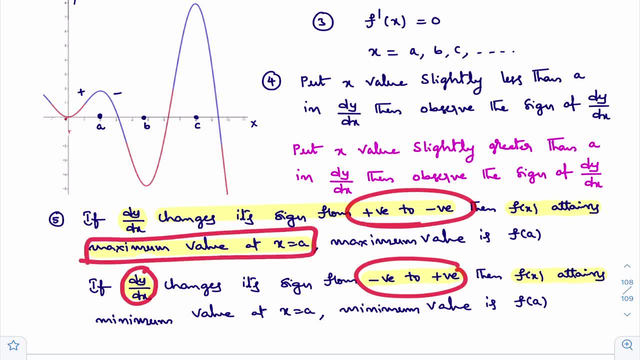 to negative. f of x attains maximum value at x equal to negative. So this is the example I explained at b. This may happen at a also. f of x attains minimum value at x equal to a and maximum value is f of a. 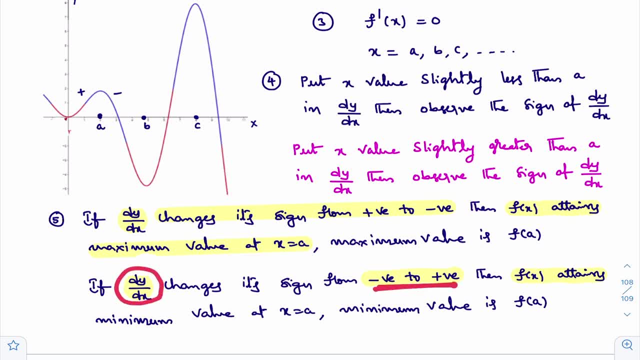 If dy by dx changes its sign from negative to positive, then f of x attains minimum value at x equal to a. Not in this graph in general, I am saying not in this graph. If dy by dx changes its sign from negative to positive, then function attains minimum. 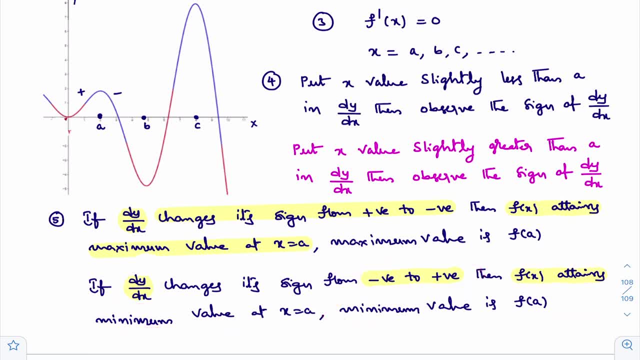 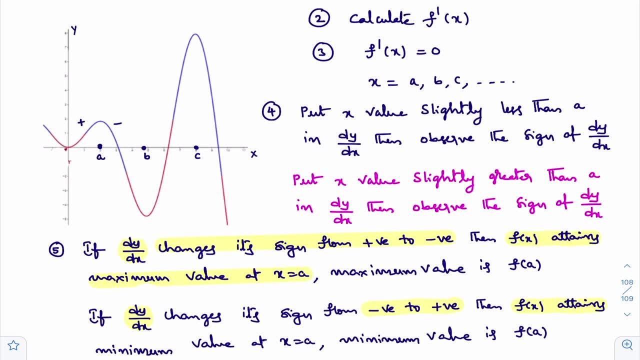 value at x equal to a and the minimum value is f of a. If I do one problem worked example related to first derivative test, Then you will get more clarity While doing exercise problems. I will do problem related to first derivative test. 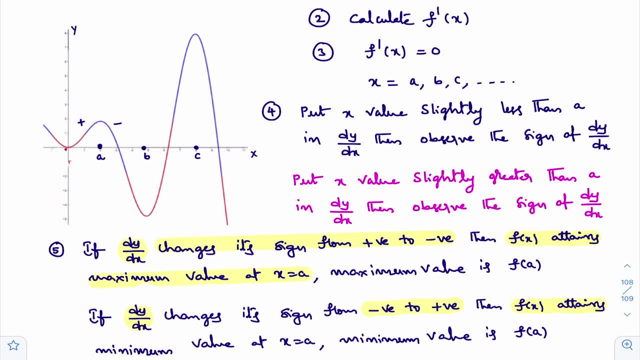 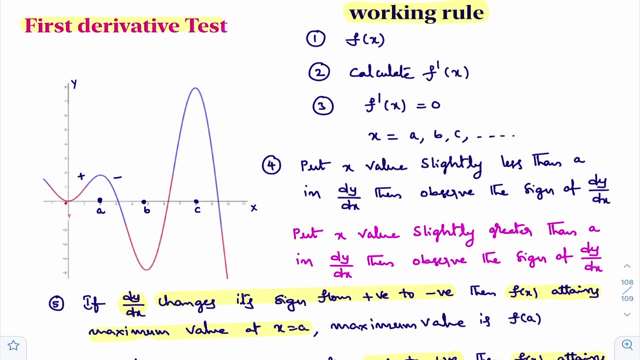 Here I checked function attains maximum value or minimum value at x equal to a. In the same way I can check function attains maximum value or minimum value at the other critical points also. So this is the working rule for first derivative test. 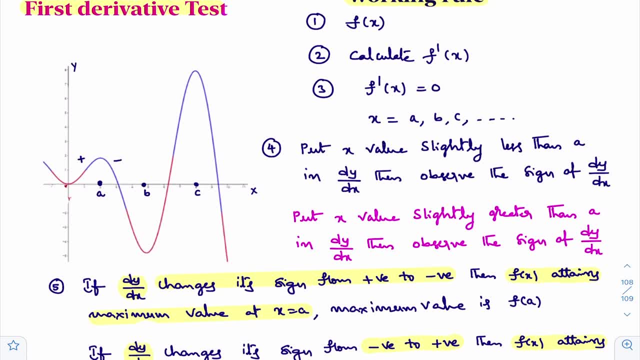 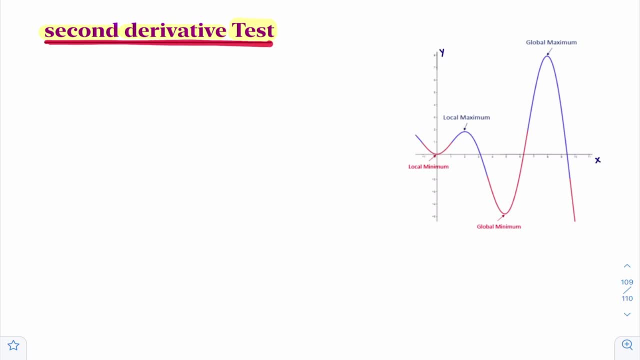 I hope you understand what is working rule of first derivative test, Second Derivative Test When we use second derivative test to identify at what values the function attains maximum values, at what value the function attains minimum value. to identify these things we will use second derivative test. 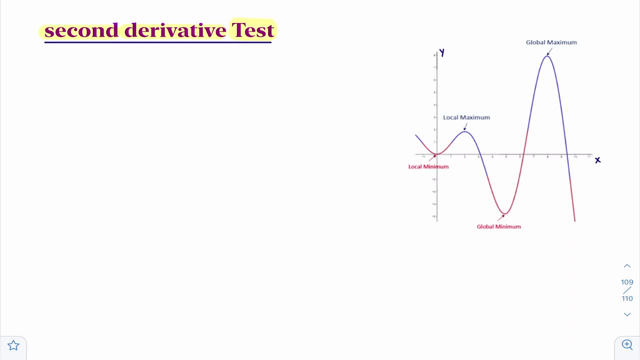 What is the working rule for second derivative test? First one: which function maximum minimum values you want to find? you take that function as f of x. So once you decided f of x, then you calculate f dash of x. How to calculate f dash of x. 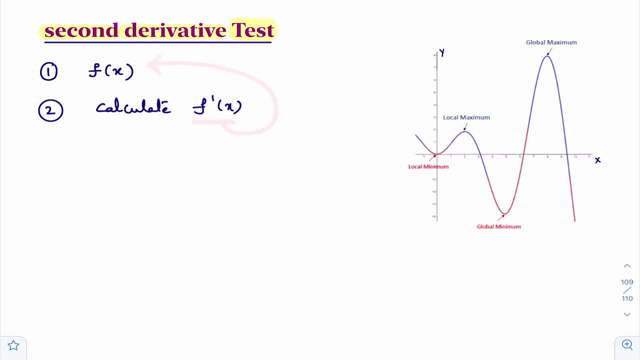 Just differentiate f of x, you will get f dash of x. After calculating f dash of x to find the critical points, you equate f dash of x to zero. Here you will get f dash of x, na you equate it to zero. 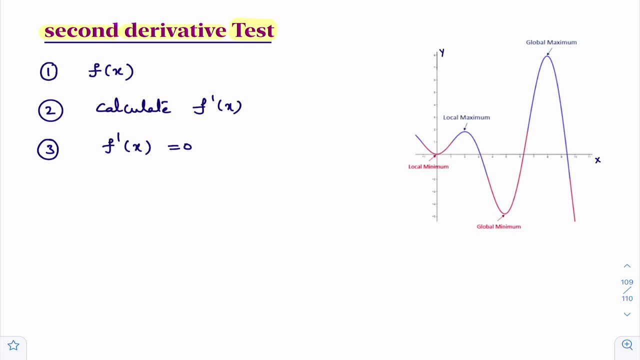 And you solve this f dash of x equal to zero, Then you will get x equal to zero. So you will get f dash of x equal to zero. So, after calculating x values like x equal to a, x equal to b, x equal to c, something, 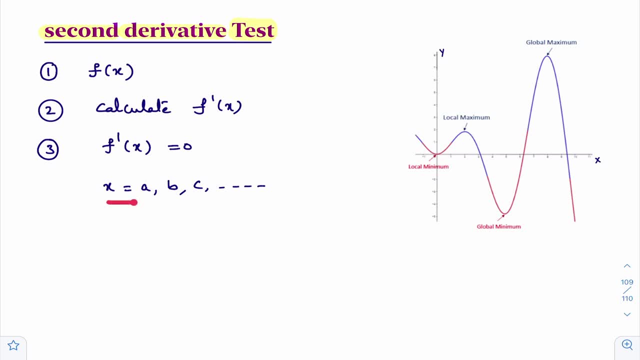 like that. you will get one or more than one value. After getting x values, you just calculate f double dash of x. Calculate f double dash of x. After calculating f double dash of x, you calculate f double dash of a. Here you got x equal to a, x equal to b, x equal to c, na. 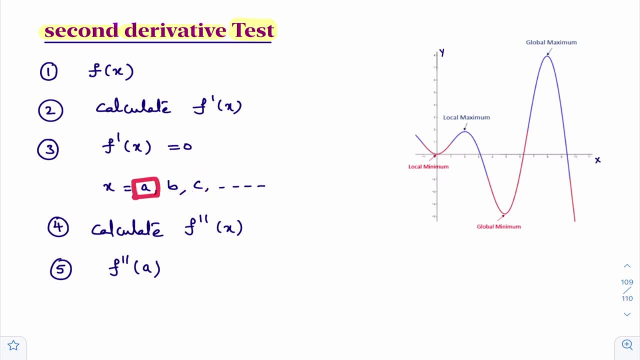 Like that: Beside at a the function attains maximum value or minimum value. you just calculate f double dash of a. How to calculate f double dash of a In f double dash of x. where x is there. there you write a, then you will get f double dash. 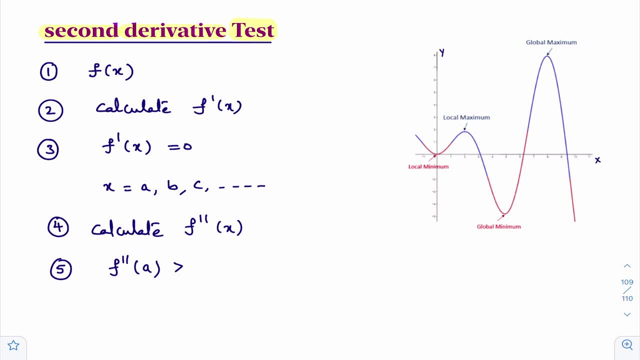 of a. If f double dash of a is greater than 0, then second derivative test says that f of x has minimum value at x equal to a. And what is that minimum value? That minimum value is f of a and the minimum value is f of a. 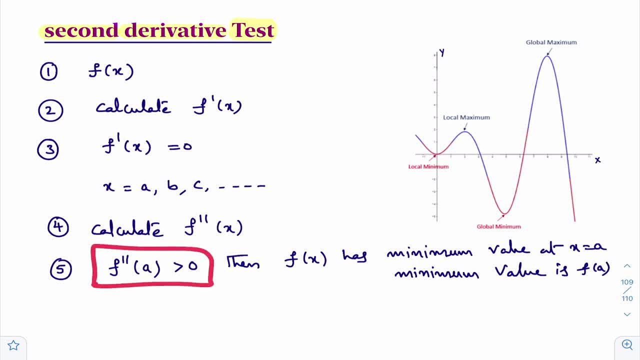 So if f double dash of a greater than 0, then we say that f of x has minimum value at x equal to a and the minimum value is f of a. In case, if you got f double dash of a less than 0, then we say that f of x has maximum. 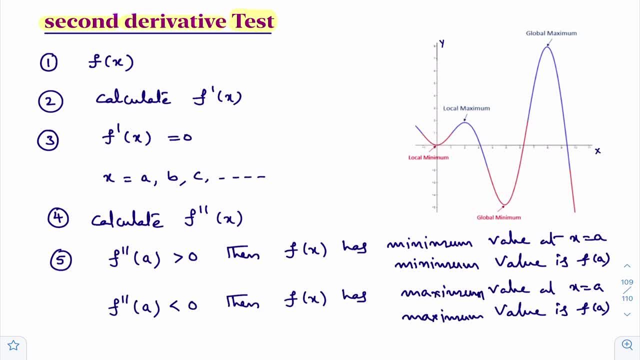 value at x equal to a. That point also I will write. In case double dash of a is less than zero, then we say that f of x has maximum value at x equal to a. you observe, when f double dash of a is greater than 0, then we are saying that f of x has minimum. 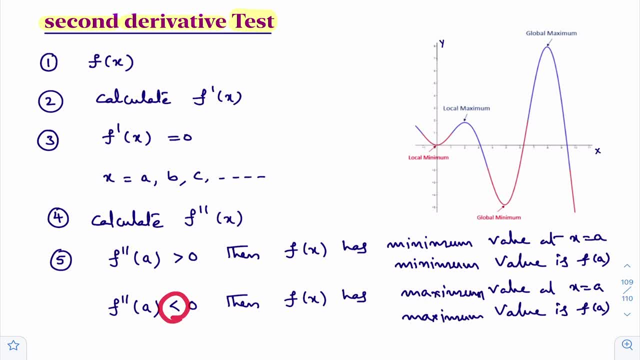 value. when f double dash of a is less than 0, then we are saying that f of x has maximum value at x equal to a. i hope you are understanding in the same way. later we will calculate f double dash of b, also f double dash of b. if f double dash of b is greater than zero, then we say that f of x has 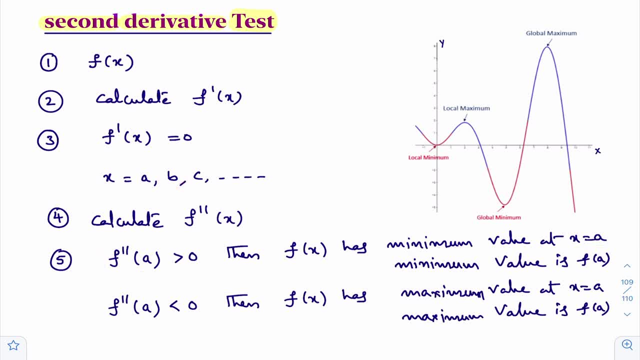 minimum value at x equal to b. in the same way, we can check where the function is maximum. what is the maximum value where the function is minimum, what is the minimum value? like that, we can calculate by using second derivative test. till now, what you learn in this theory part: you learn that 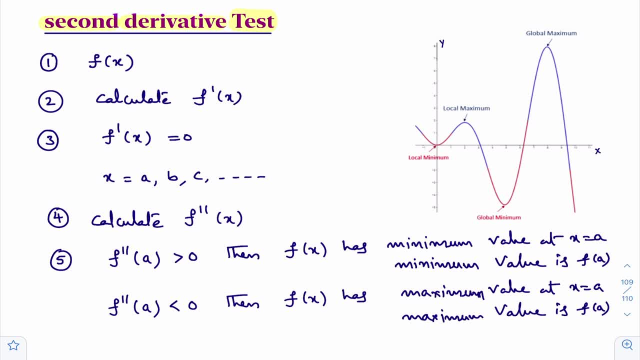 when we say the function attains maximum value. when Then we say the function attains minimum value, What is meant by local maxima? what is meant by local minima, What is absolute maxima and what is absolute minima? And to calculate where the function attains maximum values or minimum values, we use first 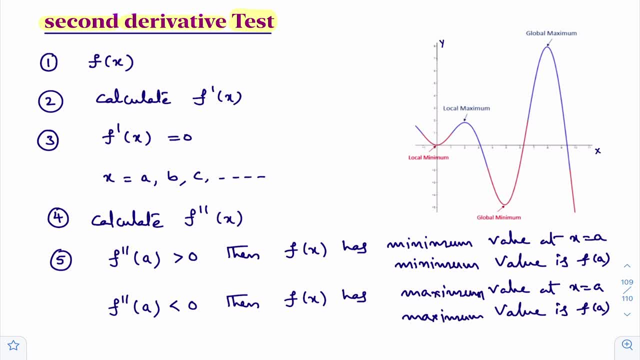 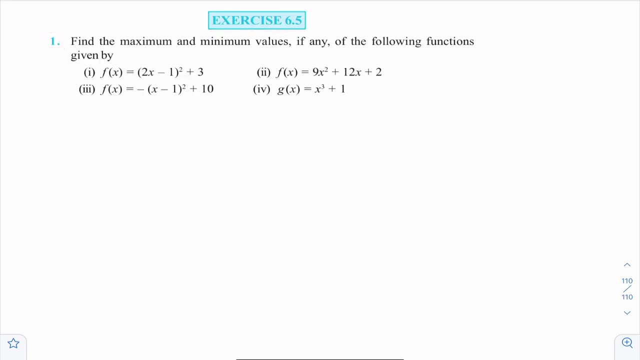 derivative test as well as second derivative test. You learned what is first derivative test and you learned what is second derivative test. In these exercise problems, most of the time we use second derivative test, Exercise number 6.5, question number 1.. 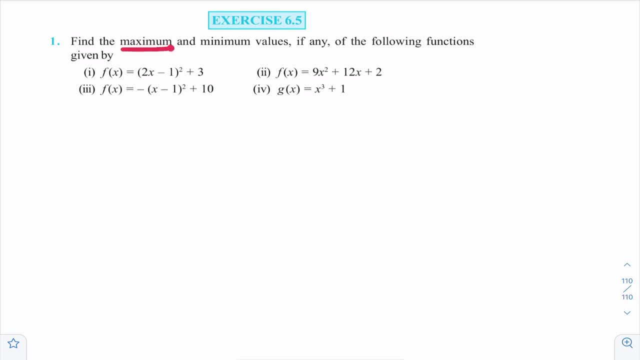 You observe the question, what they are asking: Find the maximum and minimum values of the following functions. Till now we learned theory of maxima minima, in that we identified that to find maximum values or minimum values of the function we will use either first derivative test or 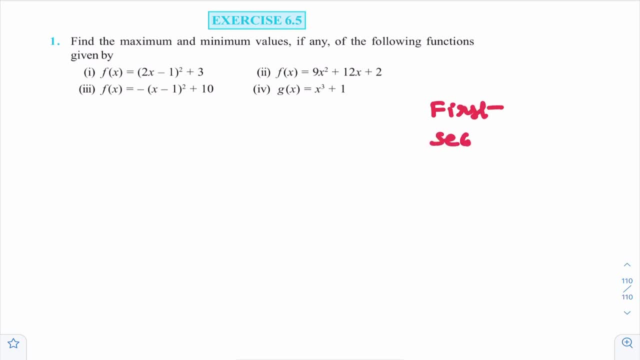 second derivative test. So here which derivative test we need to use to find maximum values, minimum values. You can use first derivative test as well as second derivative test. also, You can use any one test to find maximum values, minimum values Here most of the times. what are the problems given here in that second derivative test? 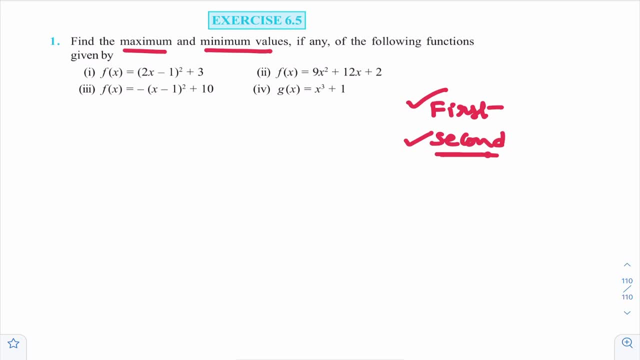 is very useful. So I will solve these problems by using second derivative test. What is the second derivative test? You see, first we will take a first bit in this. Take the first bit. This is the function. they are asking to find its maximum values, or minimum values. 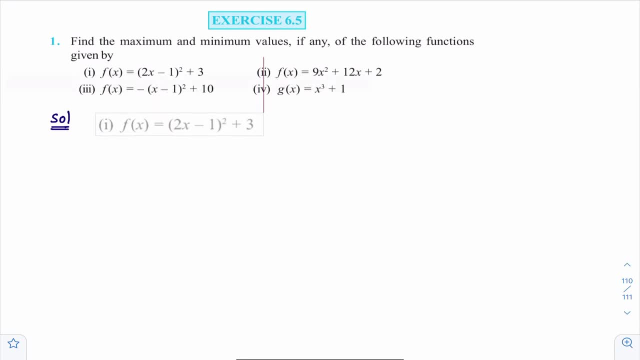 This is the function f As per first derivative test. what we need to do, we will differentiate this function. So working rule you already learned. You just differentiate this one: f dash of x. calculate f dash of x. What is f dash of x? 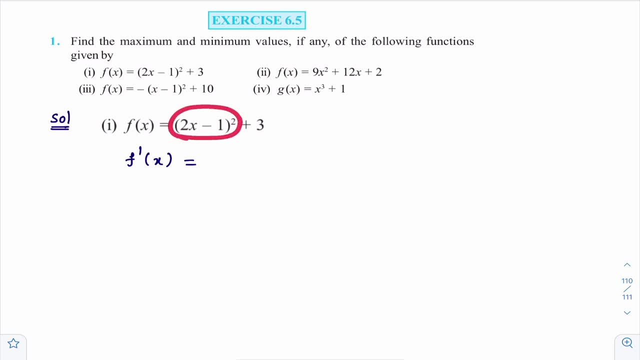 Here 2x-1- whole square derivative. we want Chain rule differentiation. you learned in differentiation chapter 2x-1- whole square. Differentiate this What you will get 2 times of 2x-1 into derivative of 2x-1.. 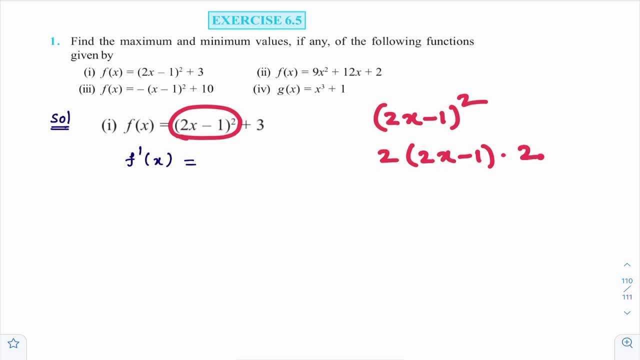 Derivative of 2x-1 is 2.. I hope you are understanding This. we learned in chain rule differentiation, So I will differentiate this 2x-1 whole square. So what you will get 2 times of 2x-1 whole square. 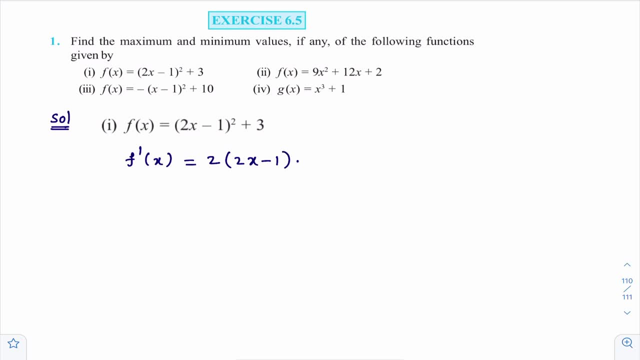 Again 2x minus 1 into derivative of 2x minus 1.. Derivative of 2x minus 1 is 2 plus derivative of constant. Derivative of constant is 0.. So you just take the given function f of x and 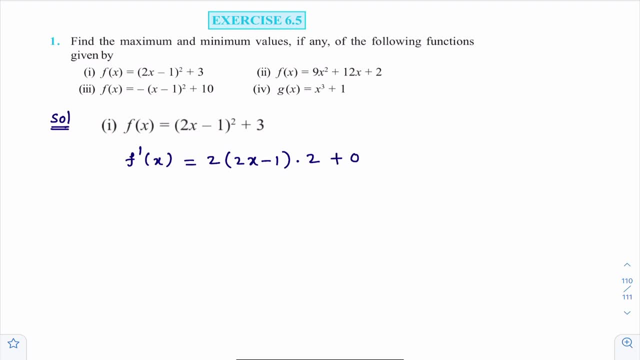 differentiate it, You will get f dash of x. You do little bit of simplification of this f dash of x. f dash of x is 4 times of 2x minus 1.. After calculating f dash of x as per second derivative: 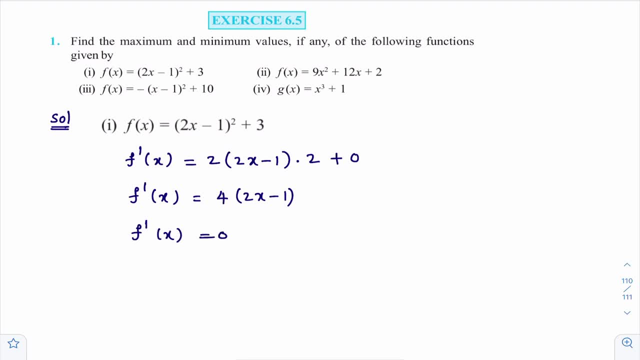 test. you equate f dash of x to 0 to find x values. You equate this f dash of x to 0 to find x values. Okay, what is f dash of x, 4 times of 2x minus 1, equal to 0.. Now you take this 4 to. 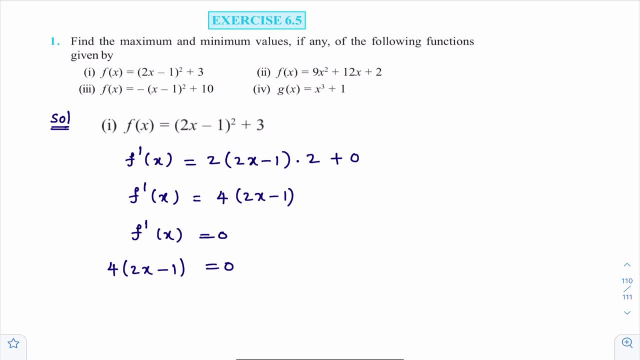 right hand side, part: 0 divided by 4 is 0.. So what you will get? 2x minus 1 equal to 0.. From this, what is x? x is 1 divided by 2.. So 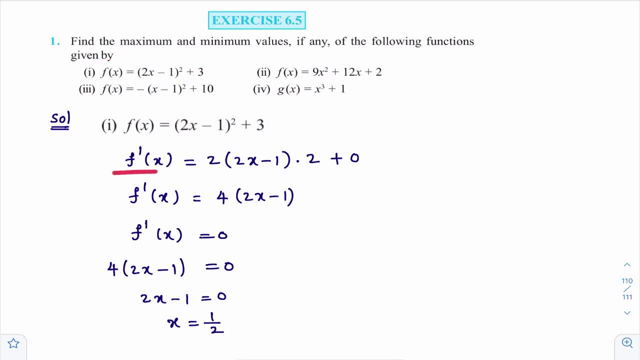 you taken this function f of x, You calculated f dash of x. After calculating f dash of x, you equate it to 0.. Now you got x values. After calculating x values, what we will do as per second derivative test, We will calculate f double dash of x. Okay, now we need to calculate f double. 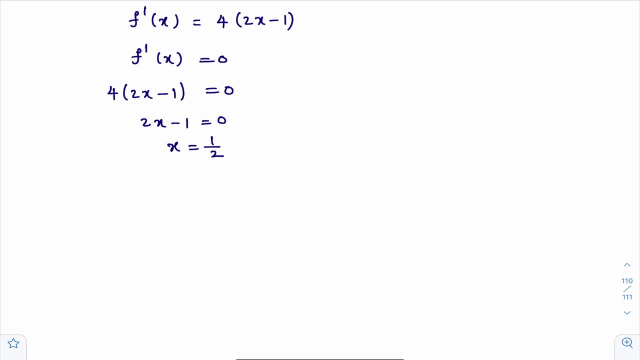 dash of x. How to calculate f double dash of x. f double dash of x can be calculated from f dash of x. You observe, f dash of x is here. You differentiate this Derivative of f dash of x is f double dash of x. Okay, now you need to differentiate this part. Okay, this is nothing, but you observe. 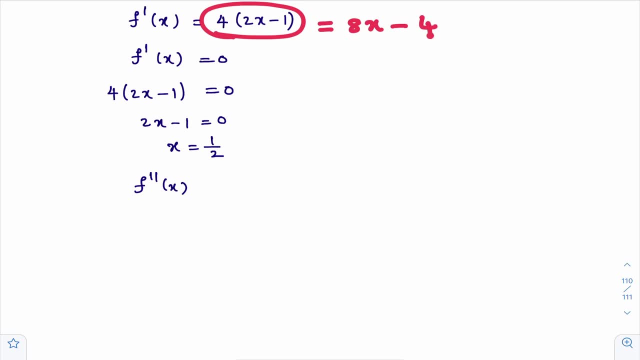 this is nothing but 8x minus 4.. Okay, you differentiate this. Derivative of 8x is what. Derivative of 8x is 8 minus derivative of 4.. It is 0.. I hope you are understanding. So what is the derivative of 4 into 2x minus 1?? That is. 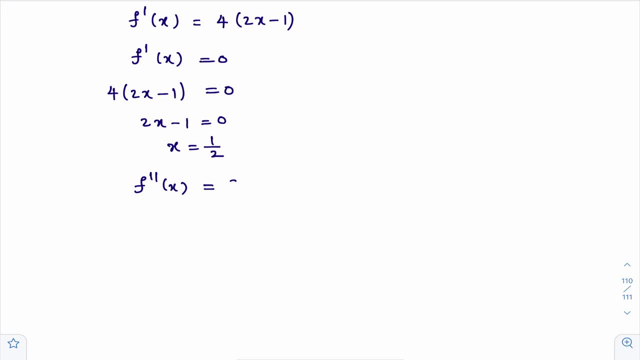 nothing but 8.. Okay, you write, it is 8.. Now you calculate f double dash of 1 by 2.. Here you see, f double dash of x is a constant number. This expression is not in terms of x, So f double. 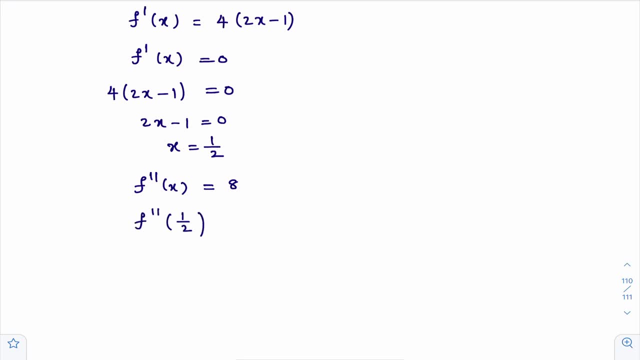 dash of 1 by 2 is what f double dash of 1 by 2 is also 8, because f double dash of 1 by 2 is also 8.. Here suppose something: x is there here, Then in place of x we will write 1 by 2.. But f double. 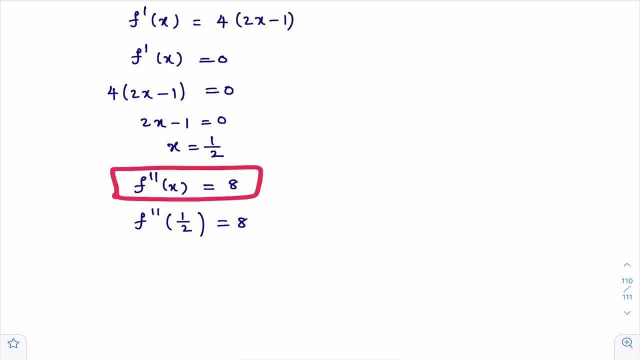 dash of x is a constant term. you got f double dash of 1 by 2 is also constant. So you check that f double dash of 1 by 2 is greater than 0 or less than 0. You got 8 here. 8 is what 8 is greater. 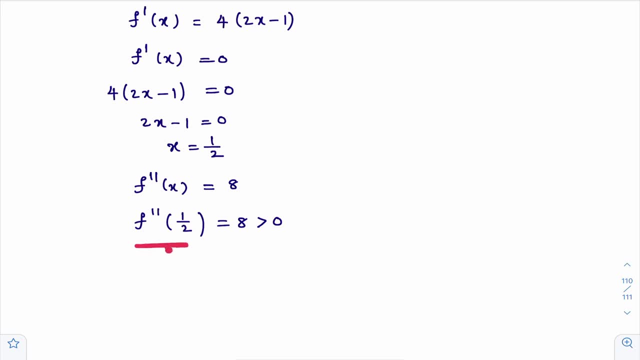 than 0. You got that: f double dash of 1 by 2 is greater than 0. From this what we can say: f double dash of 1 by 2 is greater than 0. From this what we say. We say that: 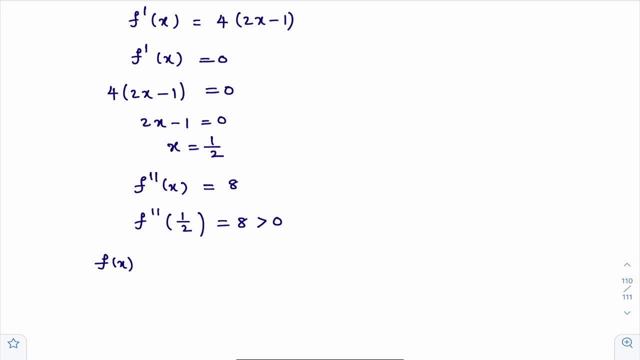 attains. we learn in the. we learn all these things in working rule, of chain, rule differentiation: f. f of x has maximum value or minimum value. f, f double dash of x greater than 0 means we say that f of x has minimum value, f of x has minimum. f of x has minimum value at where x equal to 1 by 2. 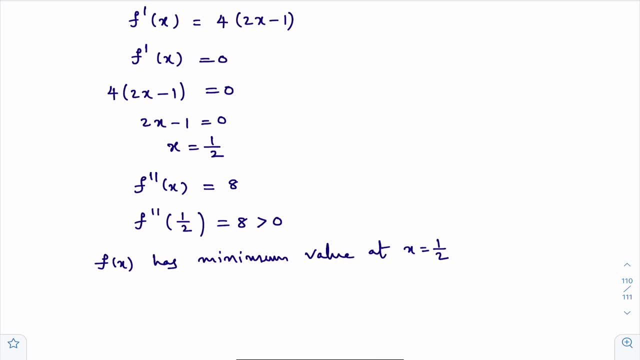 on x axis x equal to 1 by 2. is there now, at that point, the function attains minimum value. what is the minimum value, minimum value? minimum value is f of 2, f. sorry. minimum value is minimum value is 1 by 2. is there minimum value is f of 1 by 2 here? you already know f of x in this question. this is: 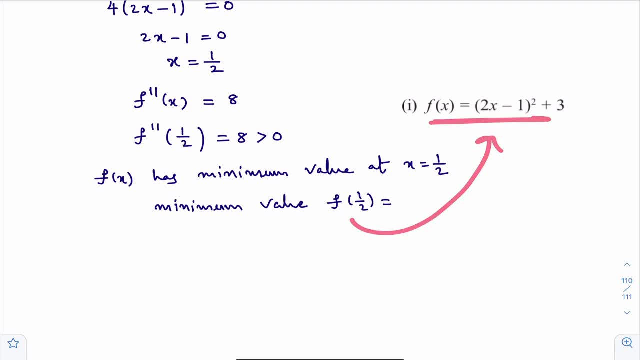 f of x. now, in place of x, you write 1 by 2. what you will get in place of x. if you write 1 by 2, 2 times of 1 by 2 minus 1, whole square plus 3, you can see here this: 2, 2. 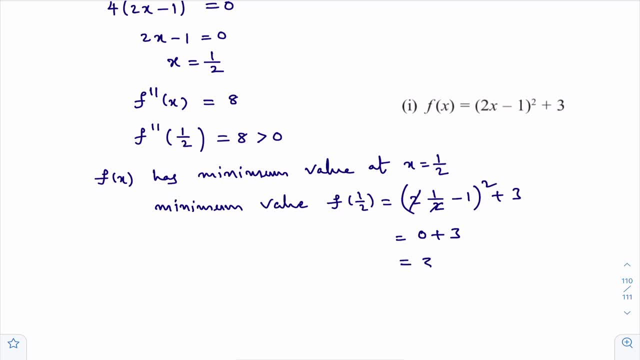 will get cancelled. this is 0 plus 3, that is nothing but 3. so minimum value- minimum value of this function- is 3 and it is minimum at x equal to 1 by 2. we can do this problem directly also, as square is there here. its minimum value is 3, but i just want you to experience the. 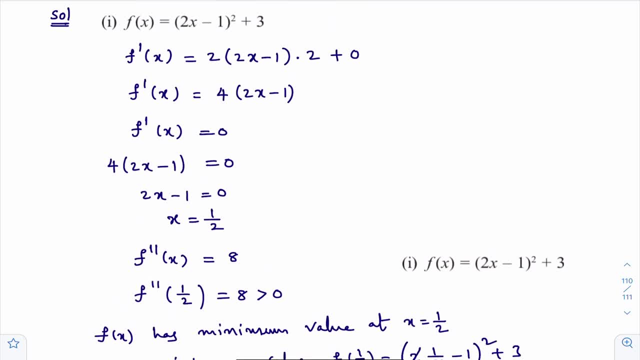 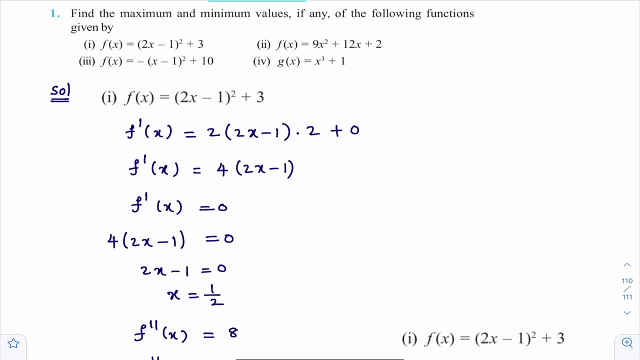 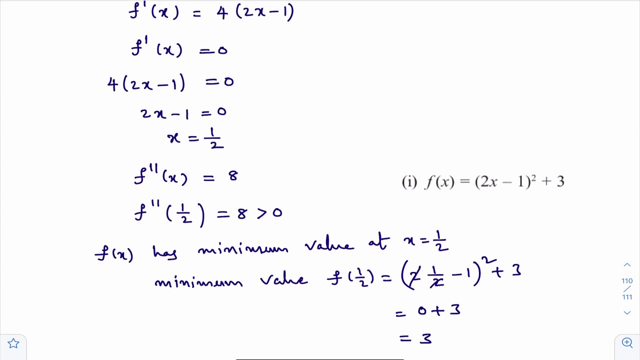 second derivative test. that's why i did this problem by using second derivative test. what they are asking in the question: find the maximum and minimum values of the following, if any exists. so here i calculated maximum value of this function by using second derivative test. you can use first derivative test also for the same problem, but i felt that 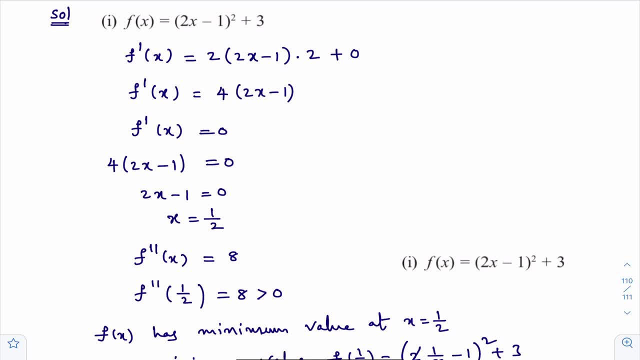 doing these problems with help of secondary interest is very easy. observe this function. second bit: in first question we need to find maximum or minimum value of this function. which one exists for this? okay, so what is the procedure? what is the working rule? they given f of x. now you take that function f of x. f of x is 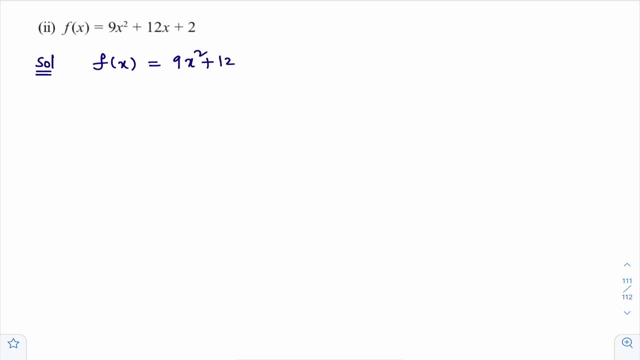 given as 9x square plus 12x plus 2. okay, what i'll do now. i'll calculate its derivative, f dash of x. okay, calculate f dash of x. 9 into derivative of x square is 2x. 9 into 2x is what 18x? so derivative. 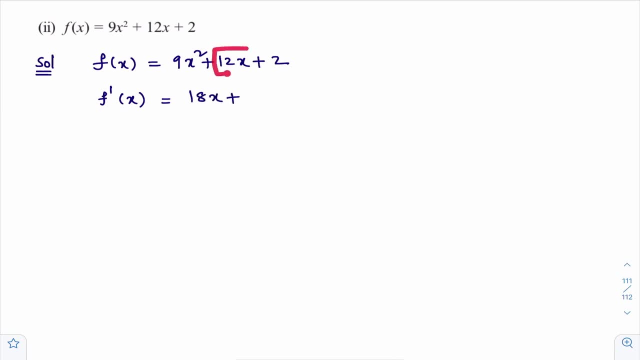 of 9x square is 18x plus derivative of 12x. derivative of 12x means here 12 is constant 12. take it outside. derivative of x with respect to x is 1. so derivative of 12x is what? derivative of 12x is 12 plus derivative of 2 is 0.. so you got f? dash of x. what is f? dash of x? f dash of x is 18x. 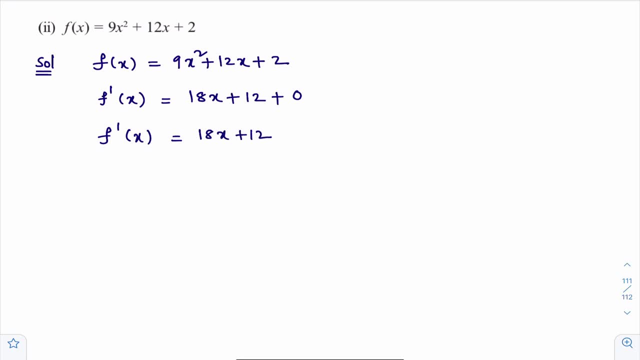 plus 12.. after calculating f dash of x, you equate it to 0. you equate it to 0. if f dash of x equal to 0, what is f dash of x? 18x plus 12 equal to 0? what is x from this? x is minus 12 divided by 18, so here: 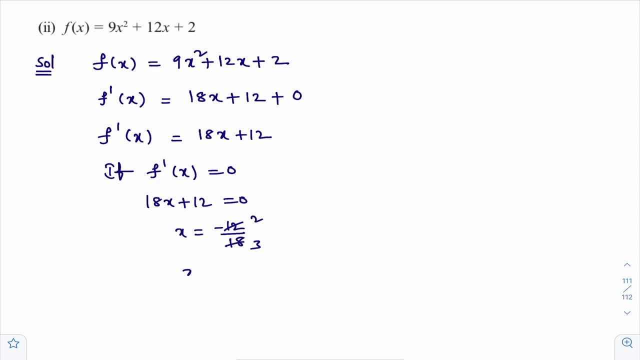 6 table 2 times 6 table, 3 times what you got, x equal to minus 2 by 3, you got, as per second derivative test: we will take the given function. we will differentiate it. you will get f dash of x. after calculating f dash of x, you will equate f. 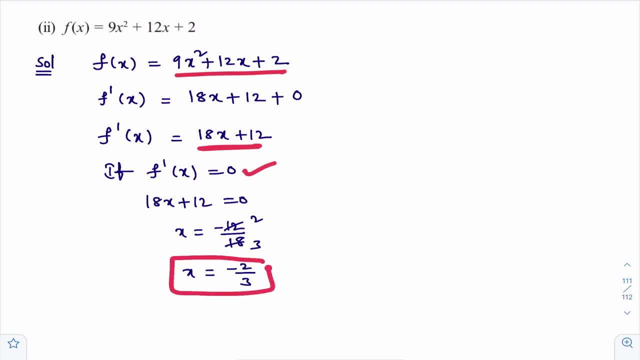 dash of x to 0, then you will get x values. here we got only one x value. after calculating x values, you just calculate f double dash of x, f double dash of x. how to calculate f double dash of x here. this is f dash of x. now you differentiate it, you will get f double dash of x. 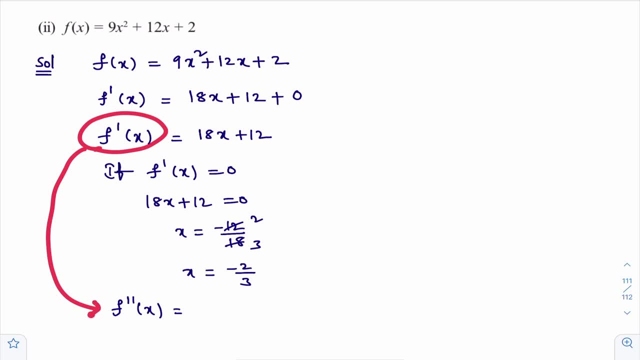 derivative of f dash of x is what? derivative of f dash of x? is f double dash of x equal to 0. now, derivative of this part. derivative of 18x: 18 is constant, now take it outside. derivative of x, with respect: x is what? 1, so 18 into 1 plus derivative of 12 is 0. now what you got, you got. 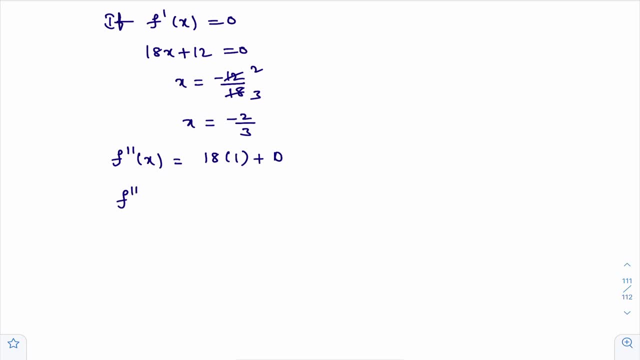 f double dash of x as 18. f double dash of x as 18. you can observe, this is independent of x. so, after calculating f double dash of x, you just calculate f double dash of minus 2 by 3. calculate f double dash of minus 2 by 3 if this is in terms of x. wherever x is there, there we will write minus. 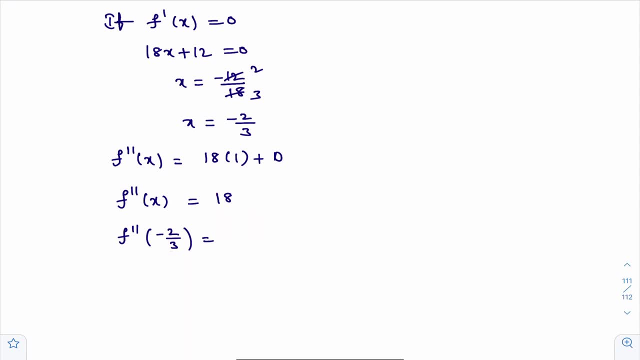 2 by 3, but this is independent of x. now this answer also: 18, only 18 is greater than 0 or less than 0. 18 is greater than 0 as 18 is greater than 0. what we will write here: f of x has maximum value. 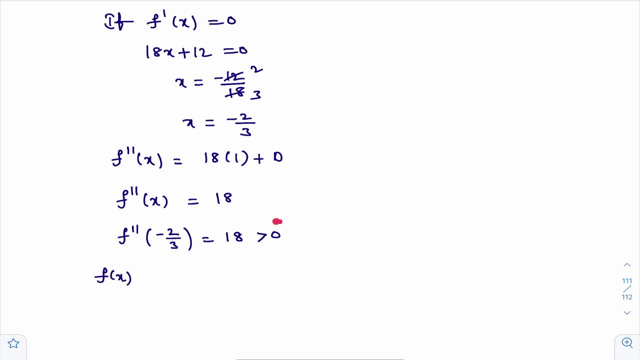 or minimum value as per second derivative test. if f double dash of x is greater than 0, we will say that f of x has minimum value. f of x has minimum value at x equal to minus 2 by 3. what is the minimum value? minimum value? minimum value is f of minus 2 by 3. now, f of x is there now. 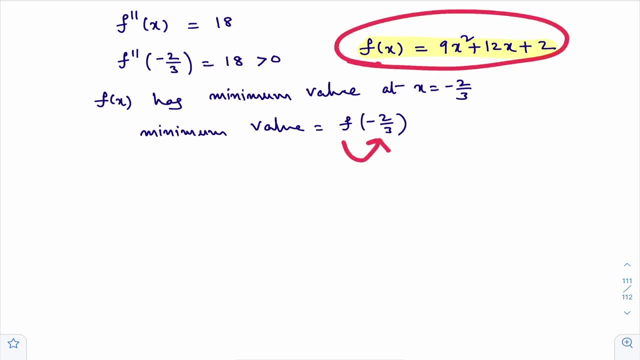 how to calculate f of minus 2 by 3, f of x already given in the question. in place of x you write minus 2 by 3, so what you will get 9 into in place of x here x square is there in place of x minus 2 by 3, right minus 2 by 3, whole square minus 2 by 3. 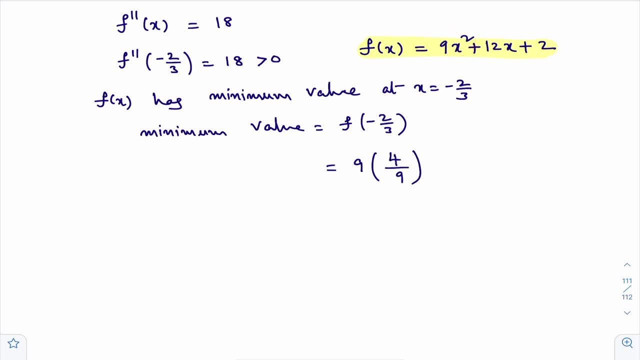 whole square is what minus 2 by 3? whole square is 4 by 9 plus 12 into minus 2 by 3 plus 2. okay, 9, 9 will get cancelled. what you will get here? 4, 3 table in this 4 times 3. 4's are 12 minus 8. 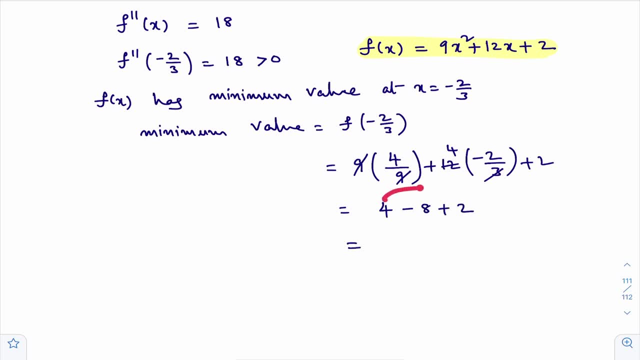 plus 2.. so what you will get here? uh, 2 plus 4 is 6, 6 minus 8 is minus 2.. so what you got here? you got minimum value as. so here for the second problem, what they are asking: find maximum and. 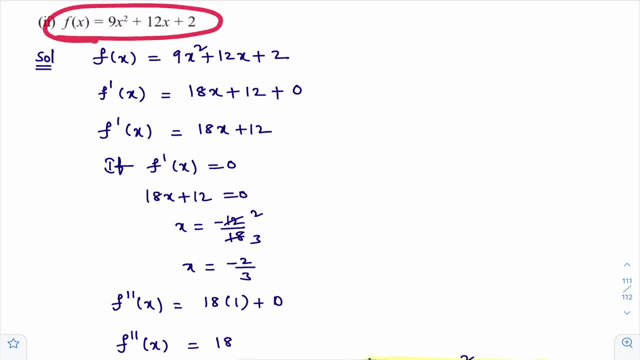 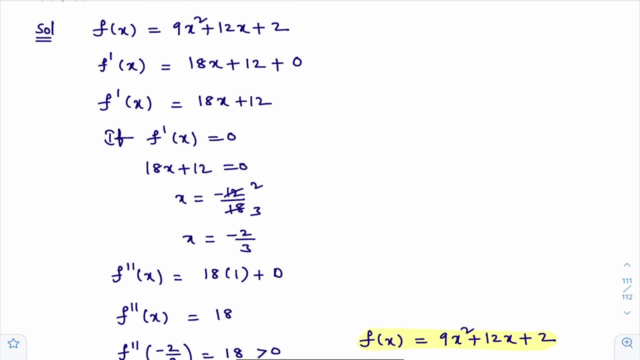 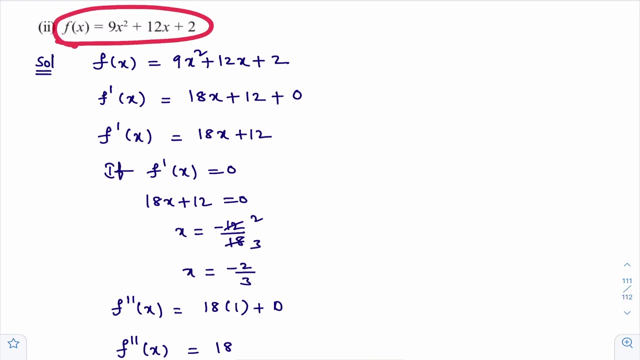 minimum values of this function. here what you got for this function, we got only minimum value. that means for this function maximum value does not exist. for that, which procedure i followed, we have to find maximum values, minimum values. one is first derivative test, another is second derivative test. 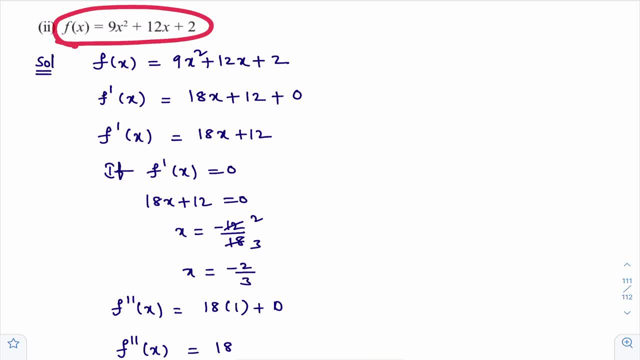 but second derivative test is easier compared to first derivatives. sometimes second derivative test is difficult. at that time we will use first derivative test. i hope by this time you are familiar with second derivative test. how to calculate maximum minimum values with the help of second derivative test. important thing is: what is the working rule for secondary value test? 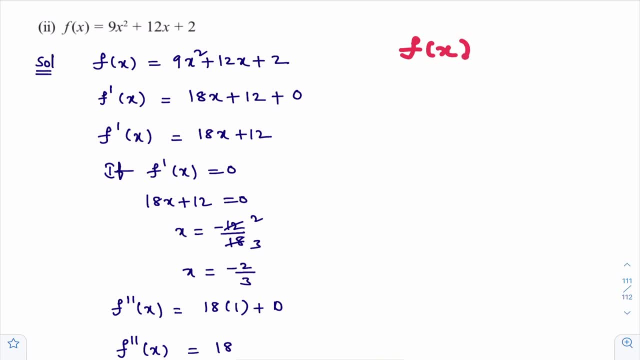 which function maximum minimum values you need to find. you take it as f of x. after that you differentiate it. you will get f dash of x. after calculating f dash of x, you equate it to 0. then you will get x values. after getting x values, you just calculate f double dash of x. 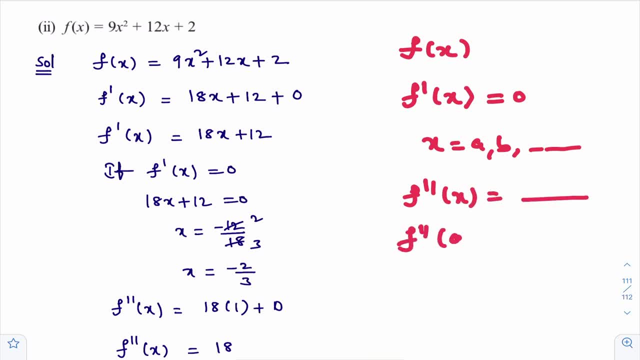 after calculating f double dash of x, you calculate f double dash of a, f double dash of b, like that. you check that f double dash of a is greater than 0 or less than 0. if f double dash of a is greater than 0, then f of x attains minimum value at x equal to a and the minimum value is f of a if f double. 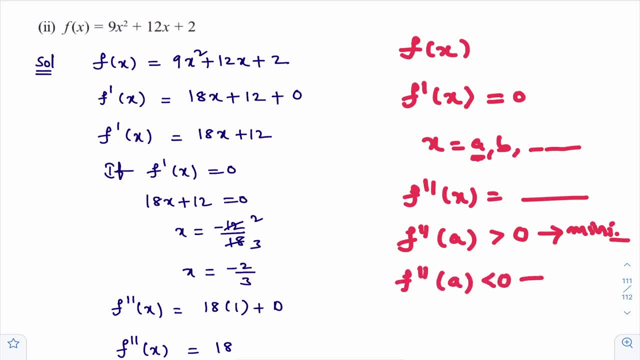 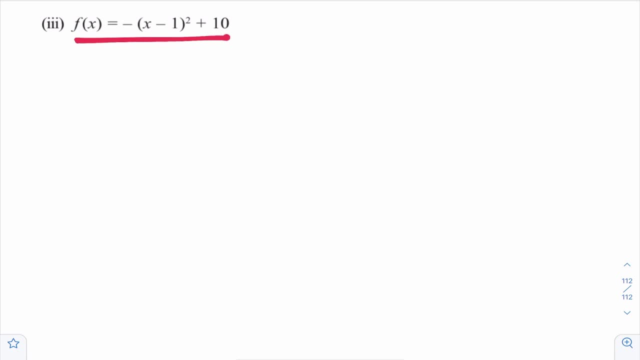 dash of a is less than 0, then f of x attains maximum value at x equal to a and the maximum value is f of a. similarly, we will check at b, c also, this is the given function, f of x. we need to find maximum values of this function, okay, first. 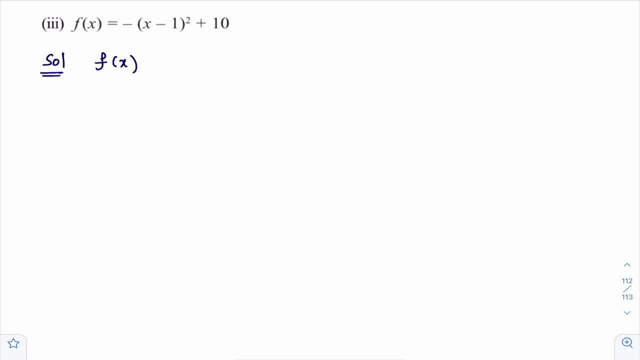 i'll take the given function- f of x is minus of x, minus 1 whole square plus 10- to find maximum values, minimum values of the function. we can use first derivative test or second derivative test. here i'll use second derivative test. in second derivative test we will calculate f dash of x. 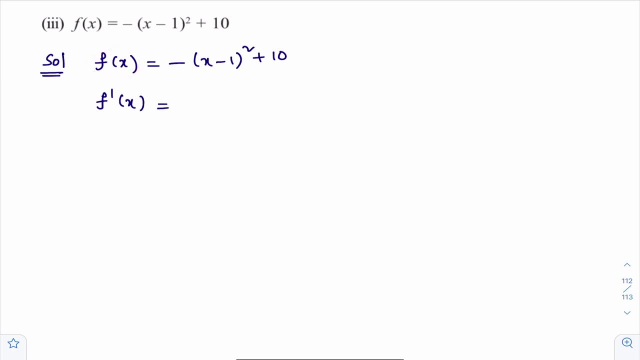 f dash of x means derivative of this function. okay, now you differentiate this. how to differentiate this here? minus is constant. take it outside. derivative of x minus 1 whole square: chain rule: differentiation: derivative of x minus 1 whole square is what 2 times of x minus 1 into derivative. 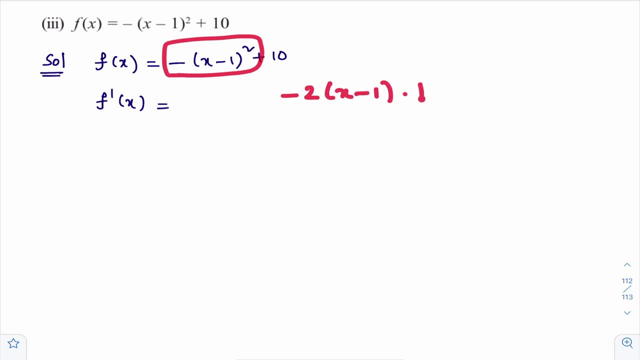 of x minus 1. derivative of x minus 1 is 1. okay, so you differentiate. this minus is constant. derivative of x minus 1 whole square is 2 times of x minus 1. whole power 1 into derivative of x minus 1 derivative. 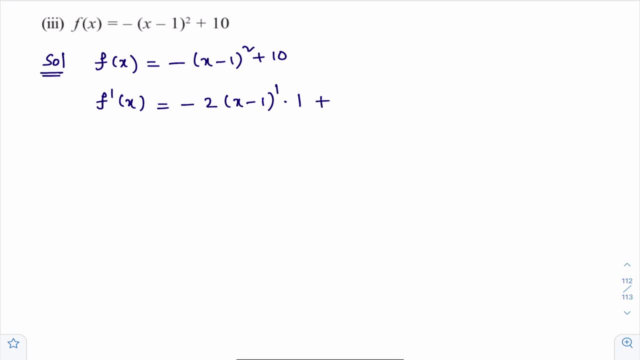 of x minus 1 is 1, plus derivative of 10. derivative of 10 is 0. okay, now, what is f dash of x? f dash of x is minus. simplify this what you will get: minus, minus of 2x, minus 2 plus 0. no need to write that. 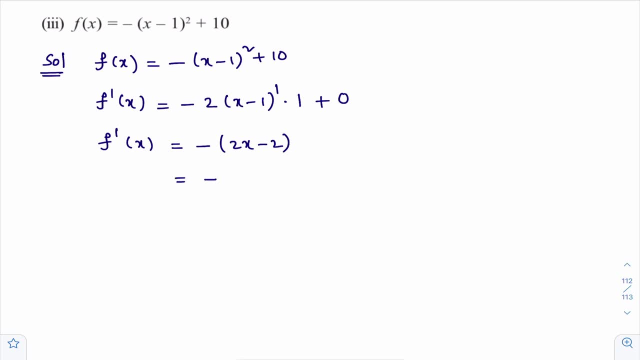 okay, if you simplify this, what you will get. you will get it as minus 2x plus 2. this is f dash of x- x. you equate f dash of x to 0 to get x values. what is f dash of x? minus 2x plus 2 equal to 0? 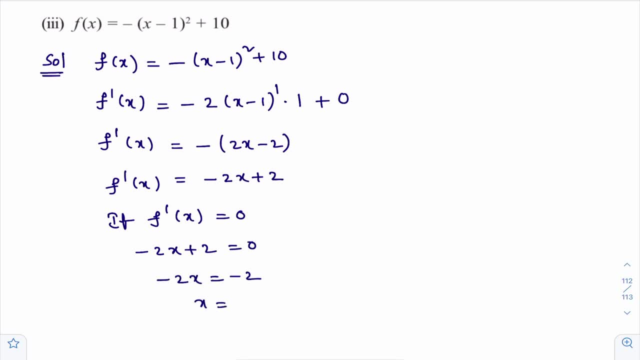 what is minus 2x from this? that is minus 2. what is x? x is 1. so you first what happened. you take an f of x, you differentiated it, you got f dash of x, you equated it to 0, then you got x values. 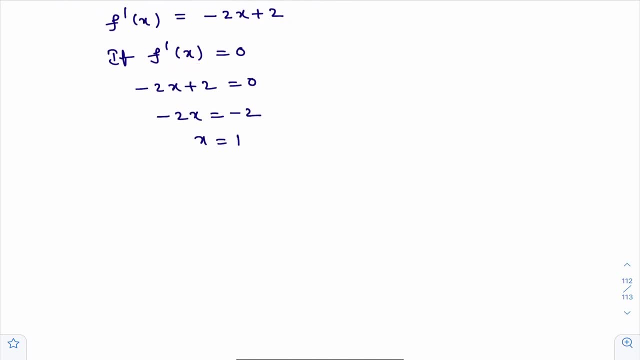 after getting x values, you need to calculate f for double dash of x. you just calculate f double dash of x. how you will get f double dash of x? you just differentiate. the f dash of x derivative of f dash of x is f double dash of x. okay, now you differentiate. uh, this right hand side part. 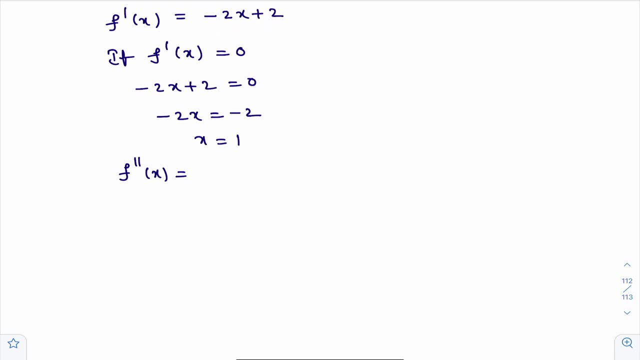 uh, derivative of minus 2x is what? derivative of minus 2x is minus 2 plus derivative of 2 is 0, right, derivative of 2 is 0.. now you got f? double dash of x, again independent of x, f double dash of. 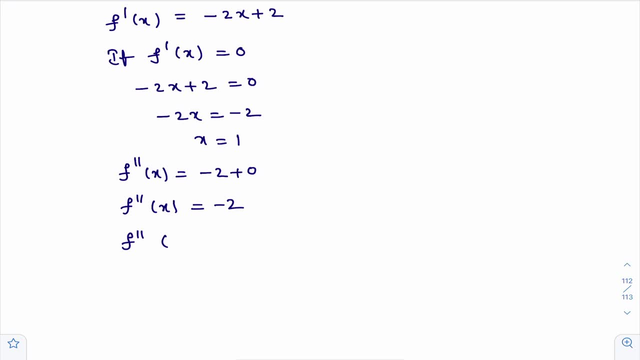 x is minus 2.. now you calculate f double dash of 1. as it is independent of x, f double dash of 1 is also minus 2. okay, f double dash of 1 is minus 2.. minus 2 is positive number or negative number, clearly. 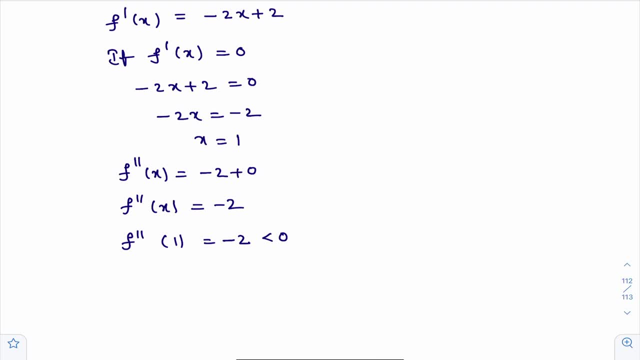 minus 2 is less than 0.. as per second derivative test, f double dash of 1 is less than 0 means f of x attains yes, f of x attains maximum value. f of x attains maximum value. f of x attains maximum value at x equal to 1.. what is the maximum value? 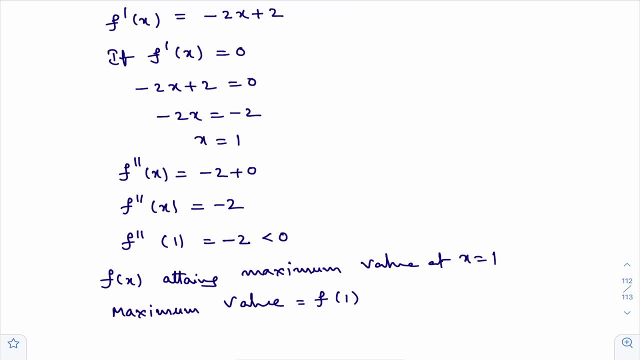 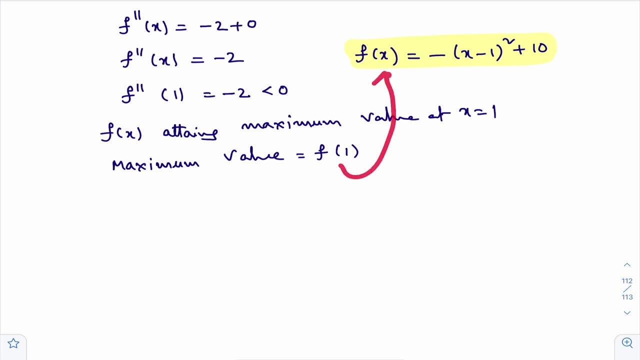 and the maximum value is f of 1. how to find f of 1? you observe, we already have f of x from the question in this. in place of x you write 1.. so f of 1 is what minus of 1 minus 1 whole square. 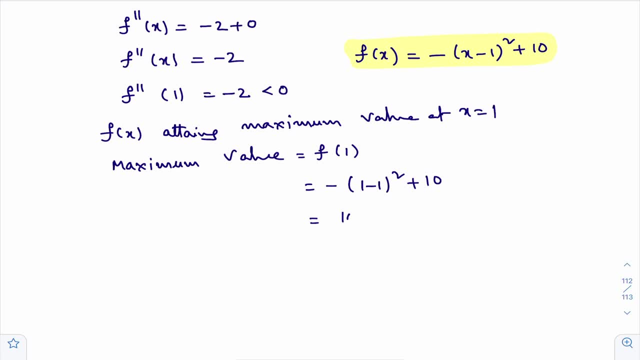 plus 10.. so what you will get this is 10. okay, so 1 minus 1 is 0 now. so you got 10.. so maximum value of this function is what? maximum value of this function is 10.. observe, this is the function g of. 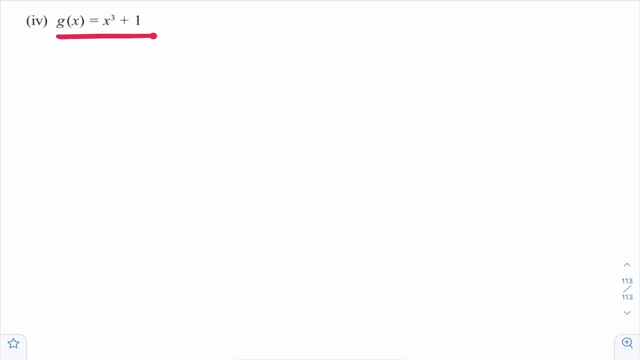 x. we need to find maximum or minimum value of this function for this problem also you can use either first derivative test or second derivative test. here i am going to use second derivative test first. you take the given function. g of x is given as x cube plus 1. you differentiate it. derivative of g of x is what g dash of x. you differentiate this right. 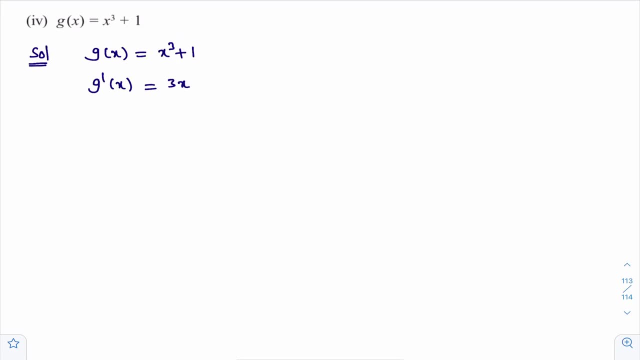 hand side part. derivative of x cube is: what derivative of x cube is 3x square plus derivative of 1 is 0.. okay, what is g dash of x? g dash of x is 3 x square. after calculating g dash of x, you equate it to zero. okay, so if g dash of x equal to zero, if g dash of x equal to zero, what? 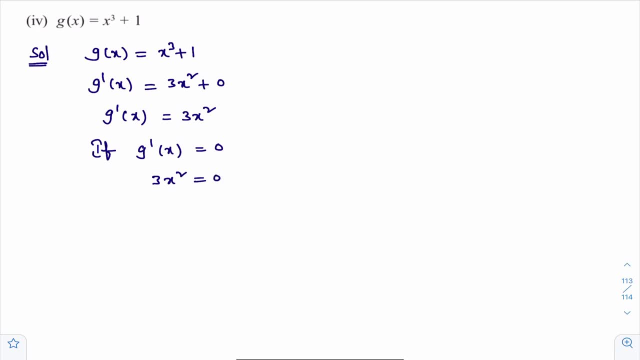 is g dash of x- 3x square equal to 0? if 3x square is 0, what is x square? x square is 0 by 3, that is 0. if x square is 0, what is x? x is 0. so, after calculating g dash of x, you equated g dash of x. 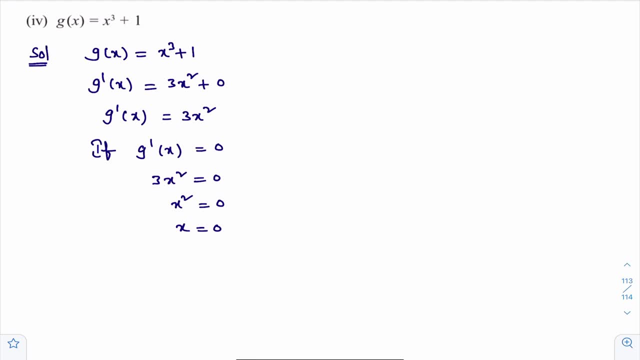 to 0, you got x values. after getting x values, you calculate g double dash of x. how to get g double dash of x? you differentiate g dash of x. you will get g double dash of x. so g dash of x derivative of 3x square 3 is constant. derivative of x square is 2x. this is 6x. g double dash of x is 6x. okay now 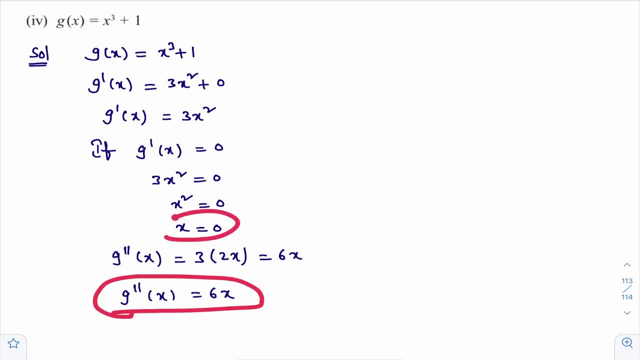 after calculating g double dash of x, you substitute this x value in this. that means you need to calculate g double dash of 0, yes, g double dash of 0. in this, in place of x, you write 0, 6 into 0, that is 0.. 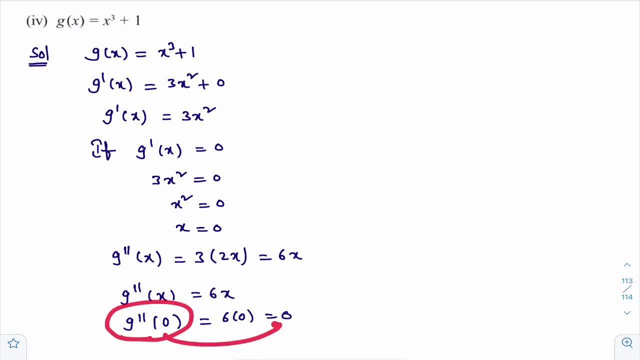 Now you need to decide that g double dash of 0 is greater than 0 or less than 0. if it is greater than 0, we can say that g of x has minimum value. if g double dash of 0 is less than 0, we can say that g of x has maximum value at x equal 0, but here you got 0. 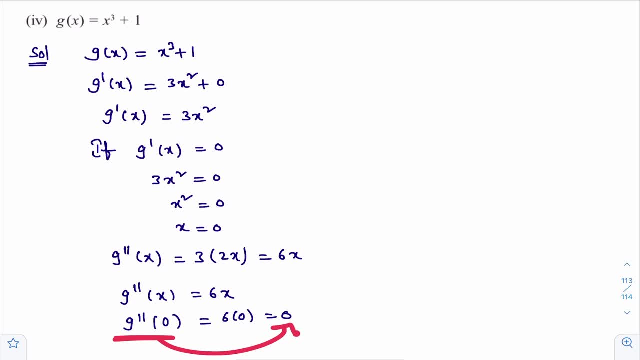 Can you decide g double dash of 0 is greater than 0 or less than 0?? this is neutral, actually. so in this case you cannot decide here g double dash of 0 is greater than 0 or less than zero. in this case we say that g of x has neither maximum value nor minimum value. 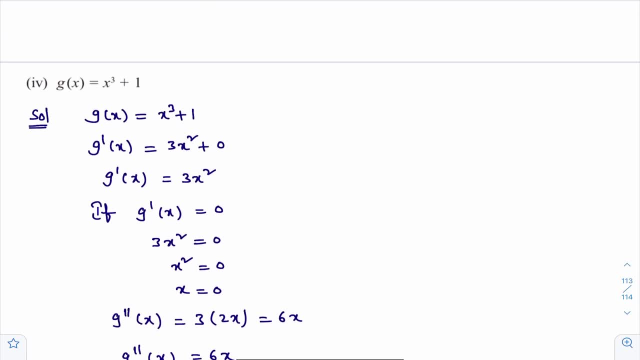 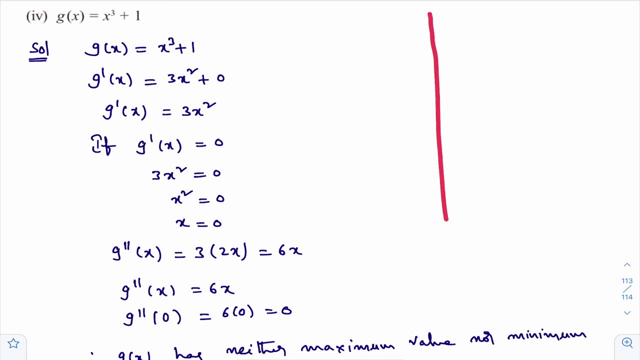 this function, g of x is given, which is not having maximum value. not having minimum value. if you observe the graph of this function, the graph of this function comes like this: see the graph of the function comes like this: this, this curve is then: this is the graph of x cube plus 1, something